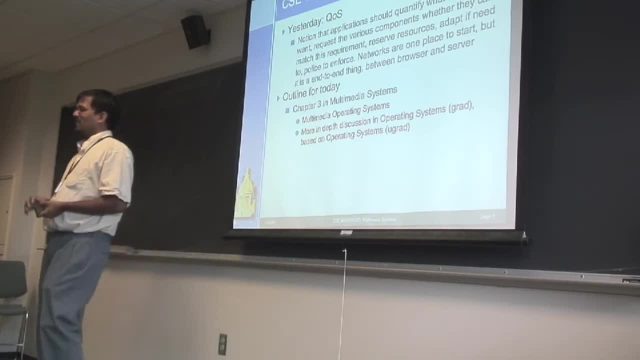 That's not their problem, right? I mean you making it free, it's your stuff, but you're taking their job, whatever, right? So I mean, but I mean that's so I don't know what's the law actually in Indiana, right? 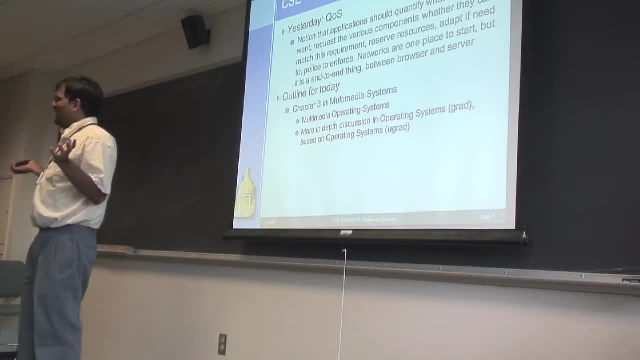 So I'm saying all this in video, but I don't know what's the law in Indiana, So it may be the case that we need to get permission. So if you ever become very popular, then I'm sure this somebody may come after this stuff, right? 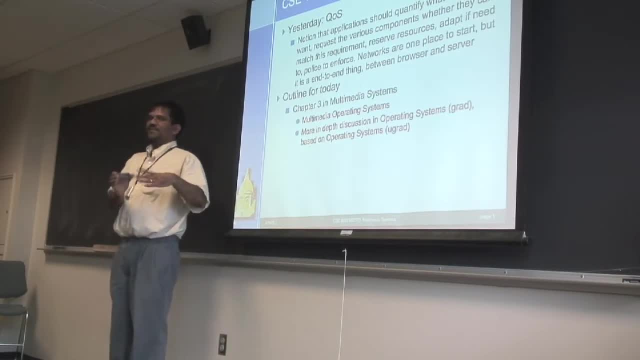 But anyway, so those are. So there are some legal issues which I don't know what the answer is for, but I'm more interested on the non-legal aspects of how this will change society, or what have you right? So, for example, if you take this video and then, like, say something, 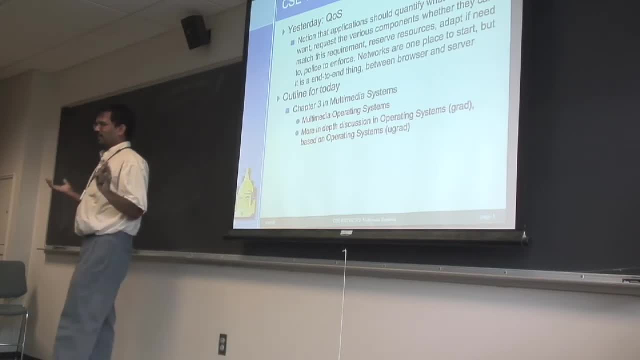 add your comment and post it on YouTube, right, And I think that's perfectly okay, but I'm not sure how well that goes in a. you know the whole aspect of it. So I still haven't graded a homework assignment. 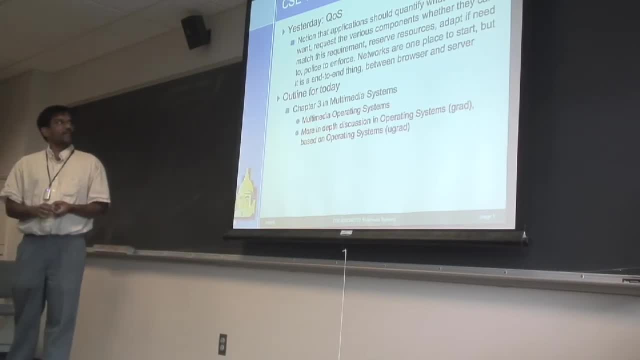 I'll probably give it on Thursday. Sorry about that. So we're going to continue back with the quality of service from the multimedia systems textbook. right, And to recap: yesterday we were talking about introducing the notion of a quality of service, and quality of service can mean different things in different levels. 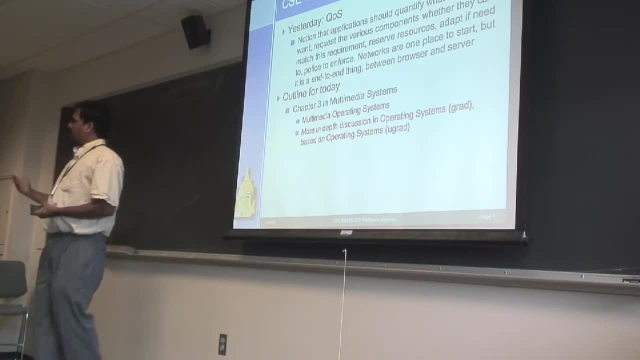 You know it could mean the perceptual, what you see. It can mean what it means to your application and the systems aspects of it. And I kind of alluded to the fact that you know it's essentially it's a really broad topic and I'm just going to give you a very high-level view. 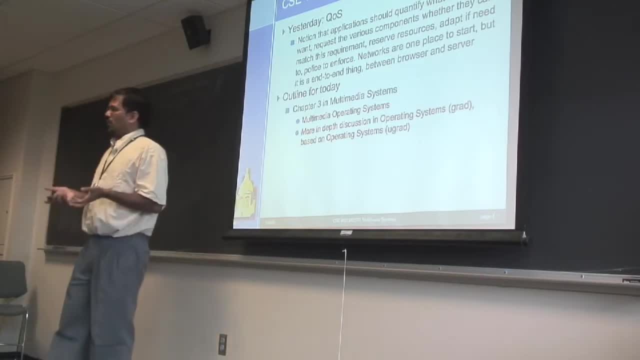 And the high-level view was: you need to be able to figure out. what is it that you want. what does quality of service mean to you? have a metric to measure it. have a metric to tell the different participants that this is what I want. 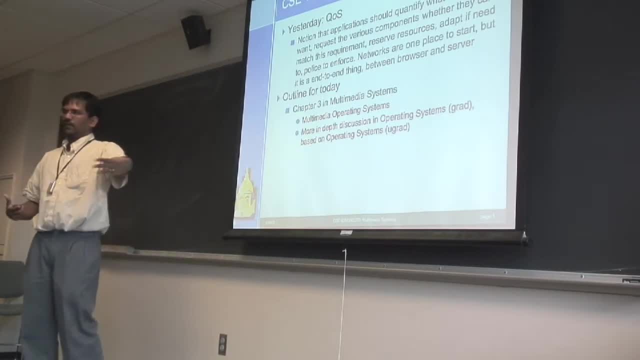 Can you give me the stuff, negotiate it, you know, hold them to what you negotiated and have it happen end-to-end right. And we kind of little talked about the network part and today we'll look more at the operating system component and what that means. 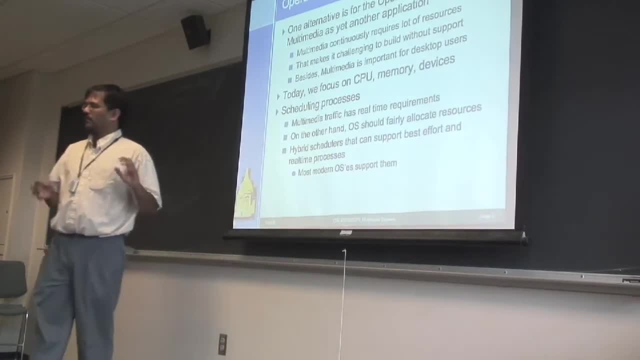 And this particular topic kind of bothered me because I like to think of myself in operating systems and multimedia operating systems. I was trying to look for good examples of research multimedia operating systems in the last six or ten years And I couldn't find any. so it sort of goes into the notion. 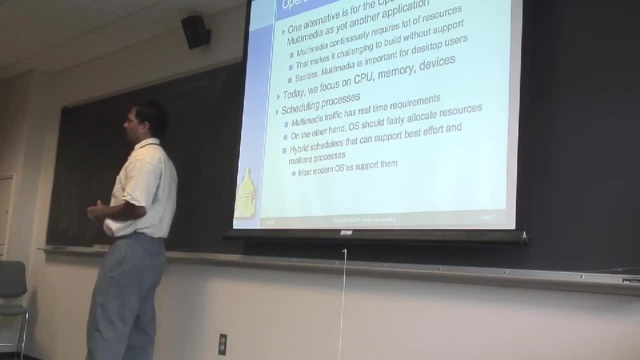 So I wanted to bring that up with the multimedia community to see what's going on. Maybe the- you know- multimedia operating system is something that we should tell our undergrads or grads not to touch because it's no longer a research thing. but there's no research going on. 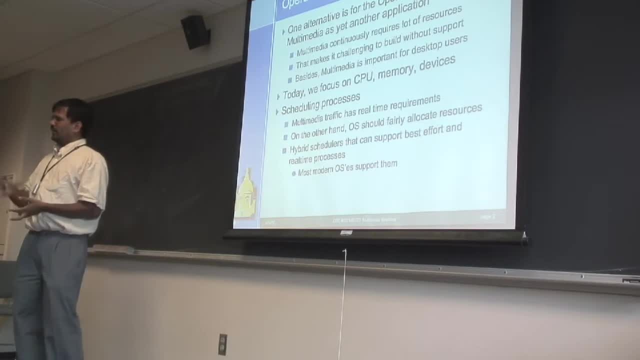 And I think I know why, but we'll leave that till the end. So the idea here again is the same thing. You know you're doing end-to-end quality of service, which means that from your application to the server and back, you want to do quality of service. 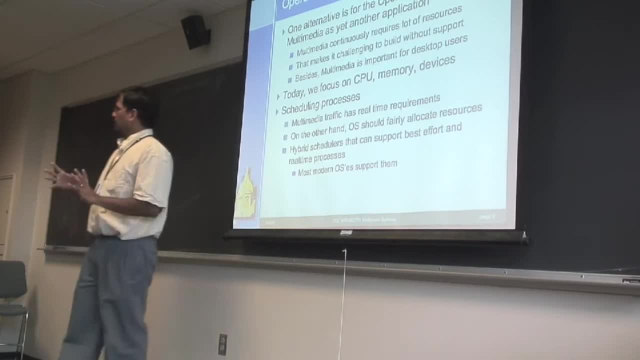 So if you sort of looked at the network aspects of it yesterday, the next aspect is to look at the operating system you know, either on the desktop or on the server, and figure out what the local machine can do to give you quality of service right. 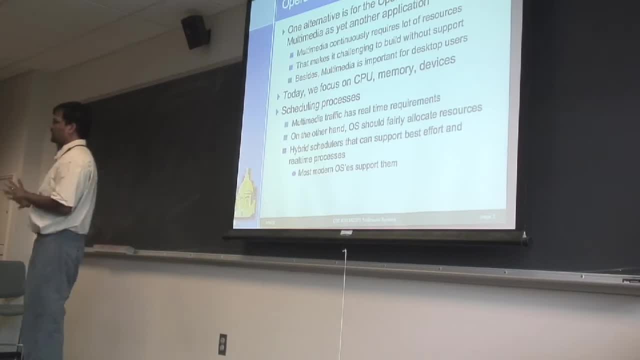 So the real aspects of it, the OS scheduling and all those things belong in another class. Unfortunately, I don't know. All of you are required to take either the grad operating system or the undergrad operating system, So you should be aware of many of this stuff. 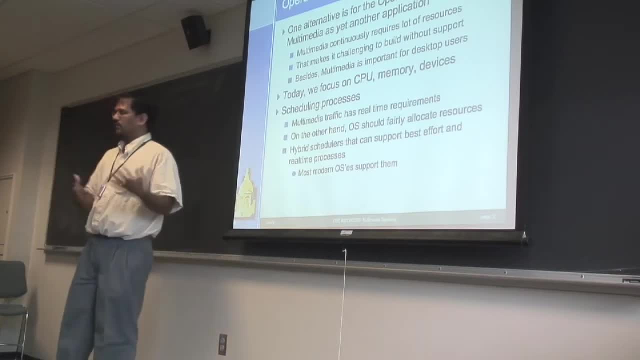 You know you spend a lot of time in trying to figure out how to schedule CPU or memory or this or what have you, and we'll look at again some of them in the context of what it means for multimedia streams. So one approach you can take is: you know, 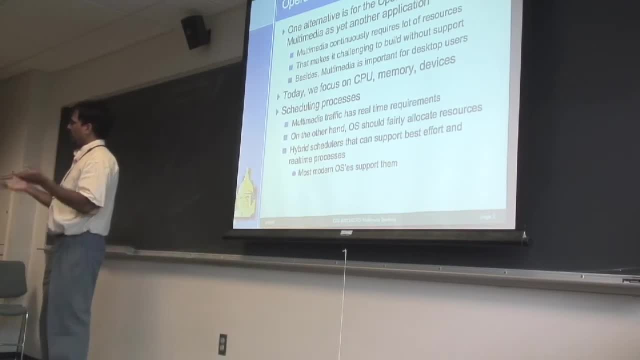 the operating system basically says the multimedia is up to you. OS should not bother You develop your applications without it knowing about it. right, And you could do that. but the problem is most of the commercial operating systems you buy out there are end up they all end up playing some sort of a media objects and that's sort 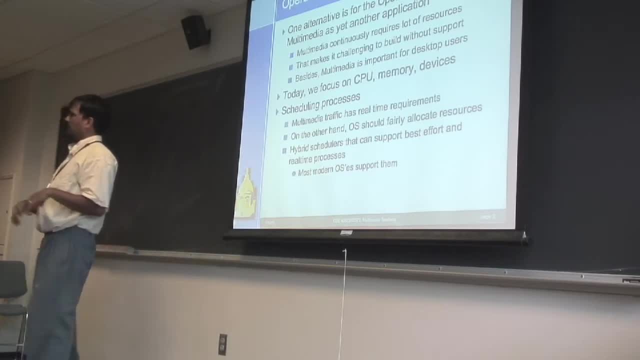 of the selling points, even for Windows XP or Vista or Mac or what have you right. So for the, at least for desktop users, they like something where they can watch a DVD or play something and sort of look good. So they demand sort of the ability to at least play right or develop little applications. 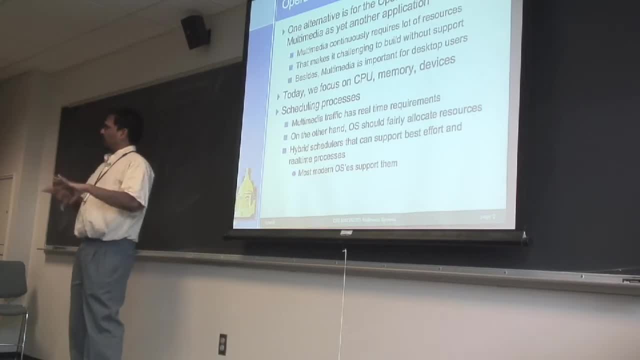 you know, like I mean, if you try the iMovie and stuff and be able to do some of these things and have them perform good, So they decide to push some of the functionality into the OS in whatever context. So we can't just say that. 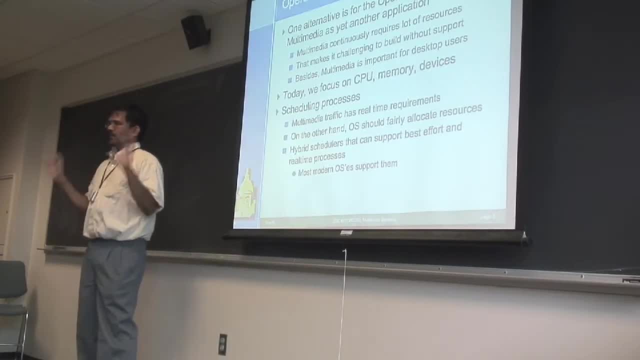 We can't just say sort of like the old Unix kind of model. It's up to you, you know, do whatever you want at the application space. So we'll focus on the three things that are locally controllable. One is the CPU, one is the memory and one is the devices. right, 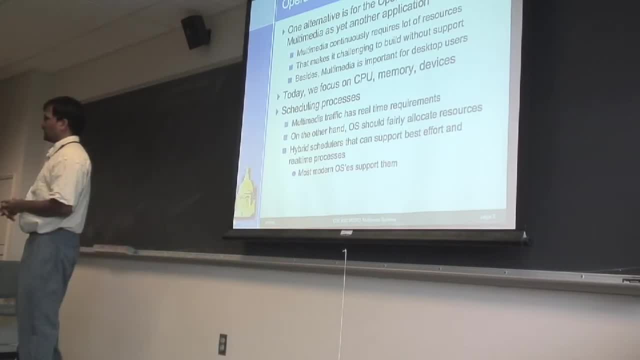 And CPU is the real-time scheduling. It's sort of what people in the real-time community would be interested in. Like we said, you know the real-time processes have resource requirements which can be quantified, So you should be able to say that to the OS what you want. 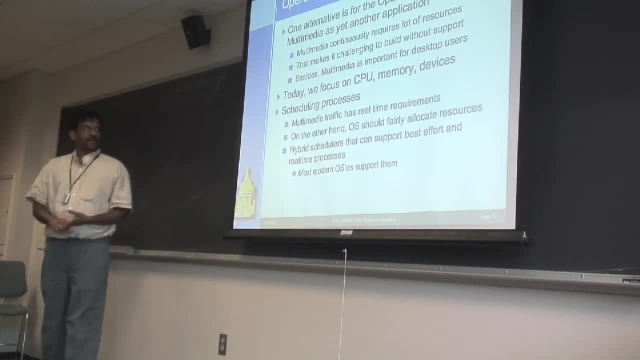 And then have the OS implement your policies right. And again we have the notion of the, whether it's the hard real-time or soft real-time, And multimedia operations tend to be soft real-time for the most part. So you should be able to tell this stuff and then get your CPU allocations. 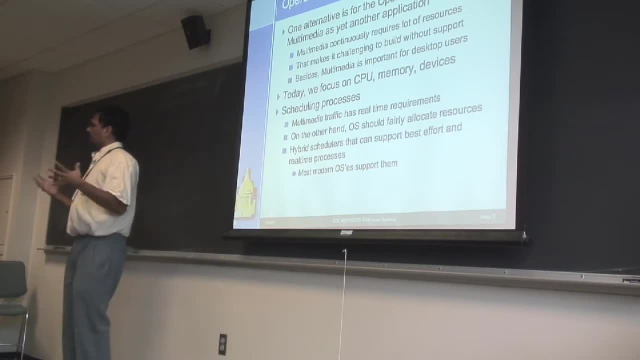 The only glitch is if you take operating systems course: right, the idea is to make it fair, whatever your definition of fair is. So you want it- the resource constraints- to be fair- Right. So you want it- the resource constraints- to be fair. 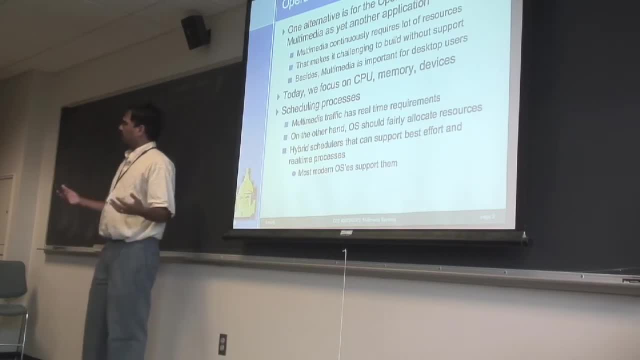 So you want it- the resource constraints- to be fair. You have to be able to divide it across the different processes on the machine, different users, or what have you, When you have this, any kind of real-time requirements, playing fair and make it useful for others? it's not that trivial, right. 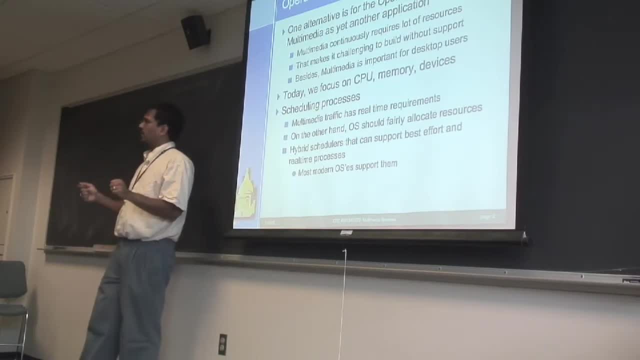 So what is fair? If I'm sitting on the console and I'm watching a DVD movie, the fair thing is to give all the resources to me so I can watch the DVD right. At least for me that's the fair stuff. 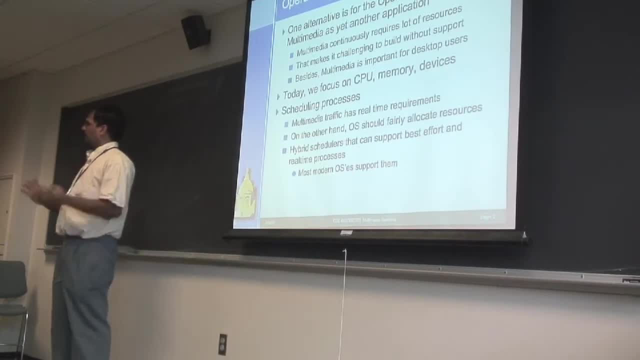 But for everybody else who's logged in remotely. that would be unfair because you're not getting any of the stuff right. So you need to kind of balance this. So from the OS perspective you don't usually talk about these balancing aspects, but from 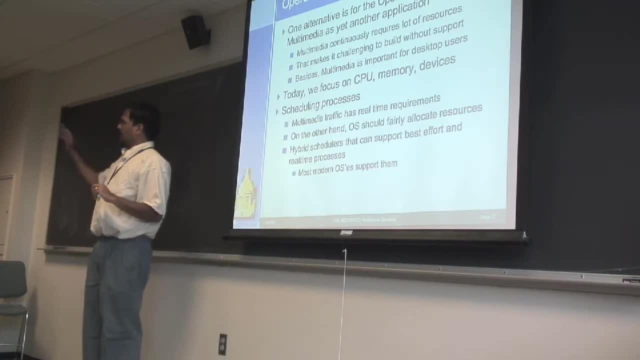 a multimedia perspective. you're going to have to give these things higher priority, higher whatever, so they can finish. So, essentially, what most operating systems tend to do is have a hybrid, like your Linux or Mac or Windows. They are pseudo real-time operating systems. 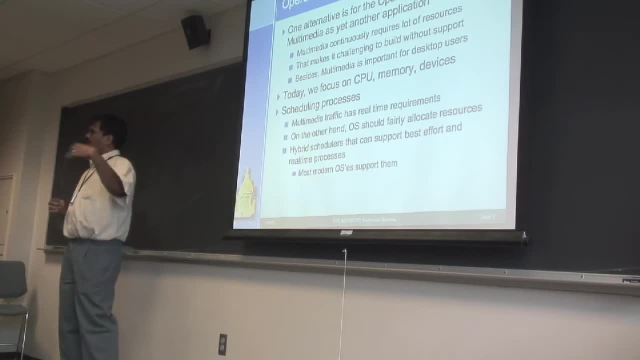 They have a notion of real-time operating scheduler. You can run your process in the real-time category and those processes don't play fair with the rest of the best effort processes and for the most part it's okay For the real-time process alone. they don't give you hard real-time guarantees, but it 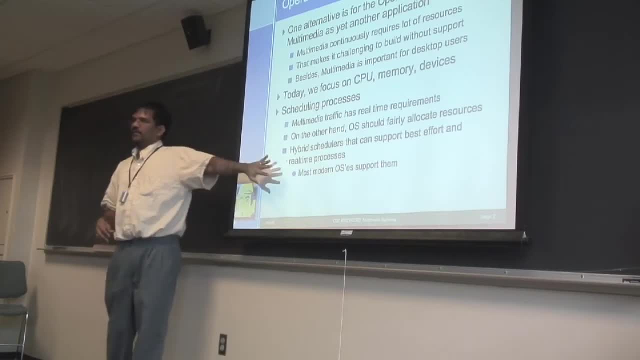 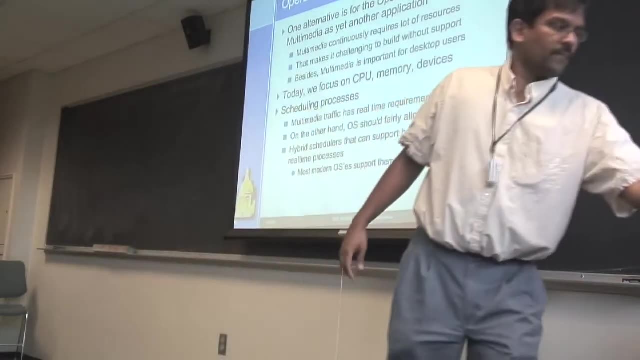 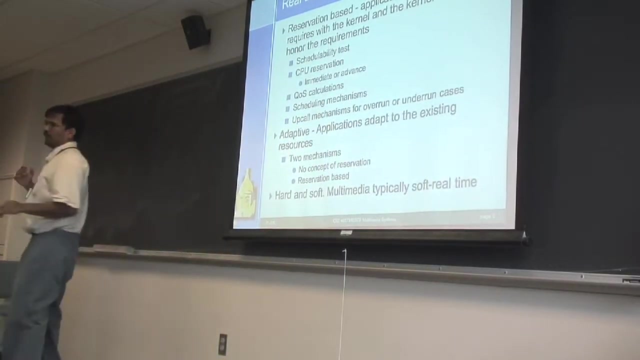 sort of tends to work out. I think that's one of the reasons why we don't see too much research, and we'll get back to that a little later. So, within the OS itself, if you were to implement this as a quality of service-based scheme, 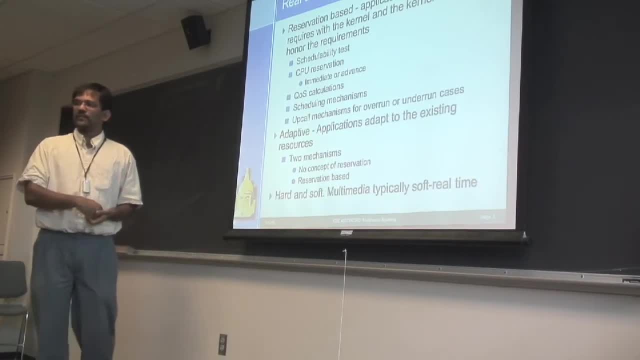 the applications ought to be able to tell the OS what kind of reservation they want. They would need some kind of guarantees so they may have to make some kind of reservation for, let's say, for CPU. It has to be a little bit more complicated than the amount of CPU I can get within an 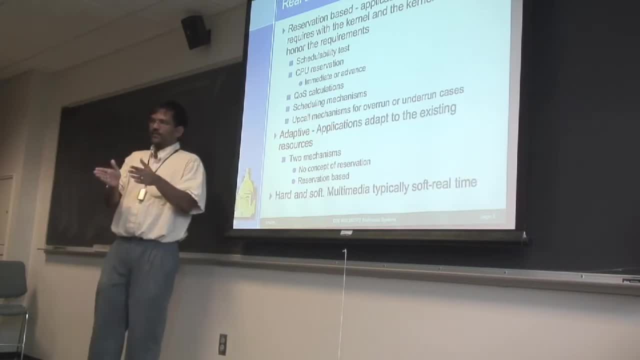 hour. They have the same kind of frames and all those things. so you need CPU in a nice fashion. You don't want to say, within an hour I want five seconds of CPU and all of them clump together. I want them in a nicely jitter-free fashion, if you can call that. 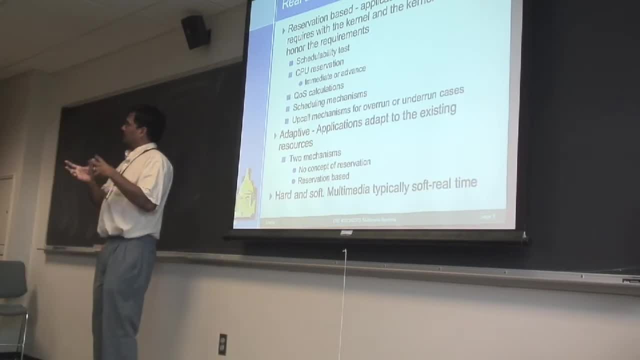 So you need to be able to define that. You need to be able to say: I want CPU where the CPU has to be. I need to schedule something every 10 milliseconds. It has to last for this much time. so I need to be able to specify not just how much CPU. 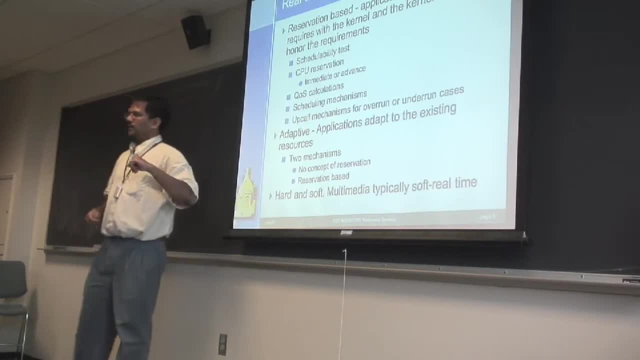 I get. So if you do that, then you still have to have a notion of schedule ability. So you have to say this to the OS. OS has to come back and say you can't run your application. You can have the reservation for immediate or for advanced use. 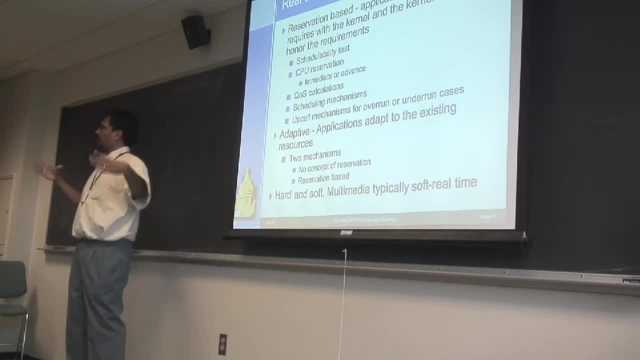 Essentially, since you're going to play something for, let's say, an hour- you're going to watch a DVD movie for an hour- you may have to make a reservation for the entire hour, which means that from now on, for the entire hour, other applications cannot come in. 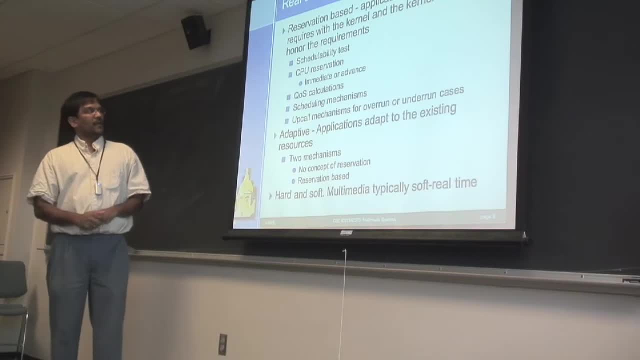 And grab resources And the other stuff we mentioned. you need to be able to reserve this. you need to be able to enforce this. you need to be able to police this, make sure that everybody's getting all the contents. You also need a mechanism to do op-call like, for the OS to inform you that it's not able. 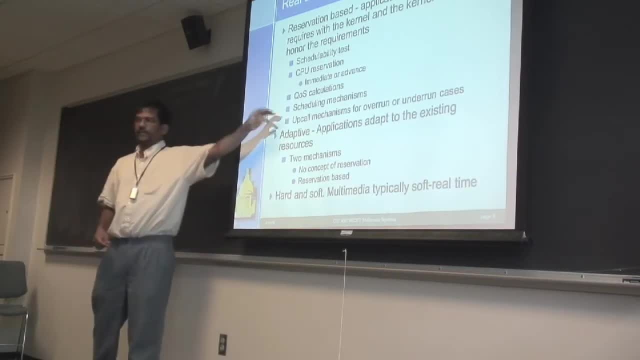 to meet the deadlines And it's essentially useful when you're doing a soft real time so you can do something about it. The doing something about it, follow-up OK, falls more into the notion of adaptive processes, So specifying and doing all these things may be hard on a desktop operating system. 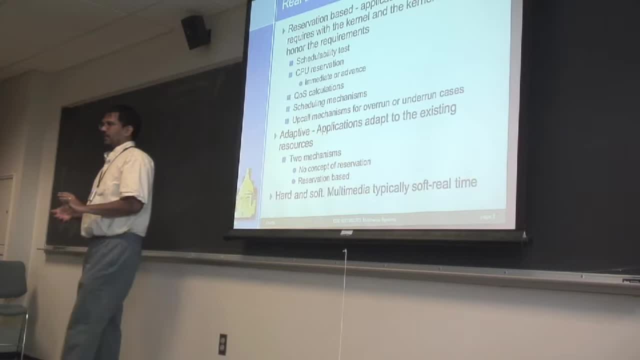 So the things you try is to make it adaptive. You try to see how much CPU you are getting and try to do your coding based on how much your CPU is getting, how much, whatever resources. You can even think of two things. One is the adaptive application has no concept of what the OS is doing, or you can still have. 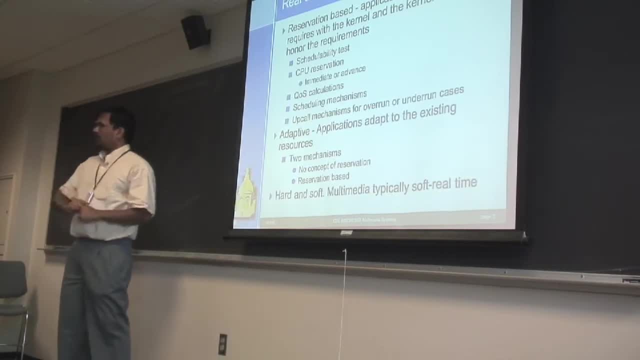 a sort of a hybrid, where you specify what you want, the OS tells you what it can give you, but you are also adaptive along the way. So you try to manage, manipulate what you're trying to do, And these are different ways to go about it. 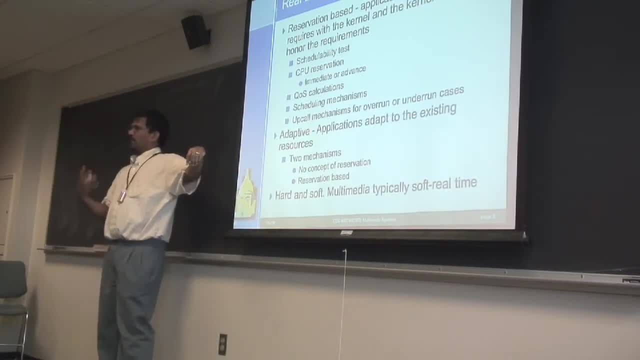 So I would think that your traditional Linux media player would be adaptive with no concept of reservation And, as you can imagine, that's not exactly a good model, Because if you're not good at it, you're not good at it. If you don't run anything else, your player would freeze up. 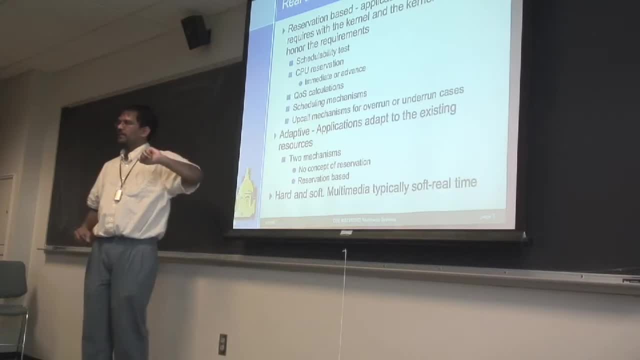 And you have various notions of this stuff. The other stuff is usually hard for you to express. Like if you're developing your own browser, it's hard for you to define what resources you need, how much you want it, express it to the OS and get the whole process going. 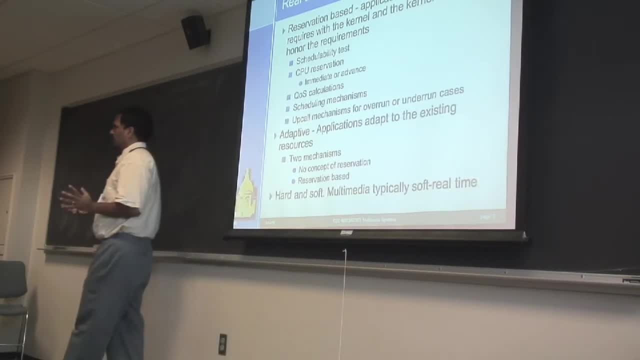 And that's one of the reasons why there are a lot of research projects which are trying to either do it automatically Or figure out how to do that. And I think we have solved it and I'll show you how some of the Mac and Windows tries. 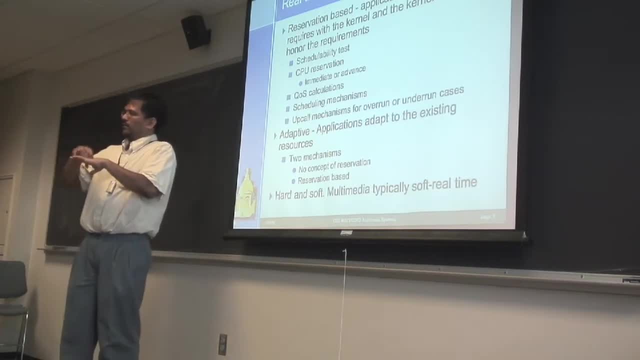 to solve that Essentially, they kind of have a library that you use and the library defines all these parameters for you and negotiates the rest of the OS. Yes, Does the Windows Media Center take care of any of this or what's involved in that? 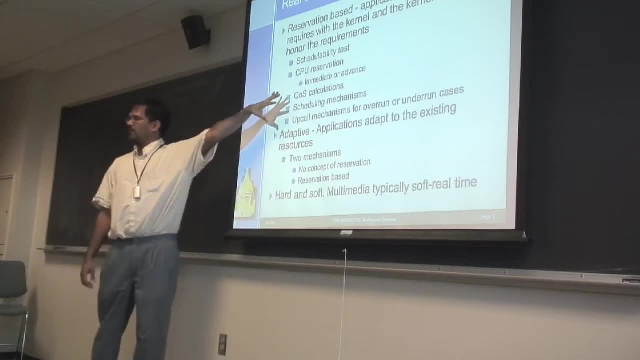 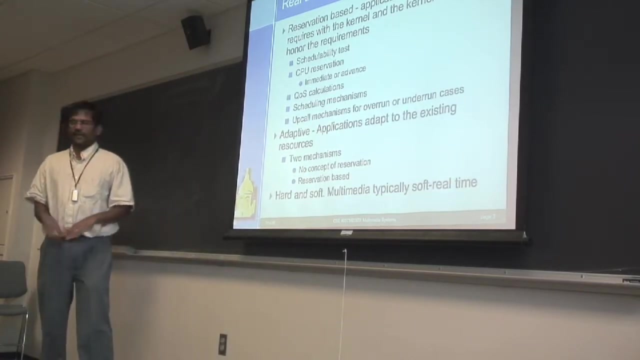 Yes, the Windows Media Center or Mac OS basically does some of this stuff. They don't do full reservation but I think they do they sort of more in the. they know how much operations you need because you open those. I'll get to that in a little bit. 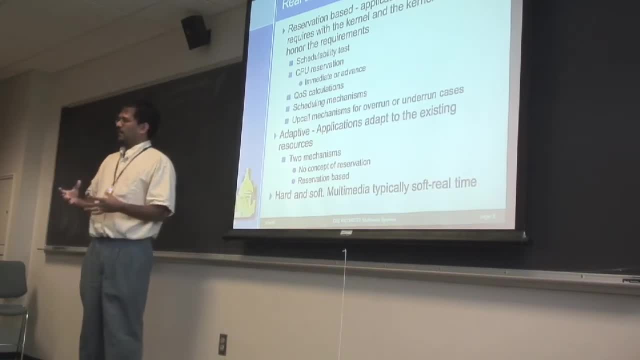 Again at a very high level, because the details are actually. the reason is the details are not forthcoming right Like either Vista does not release. I was trying to look through to see documentation. I mean, they would like to give you the API, but not what exactly they're doing to get good performance. 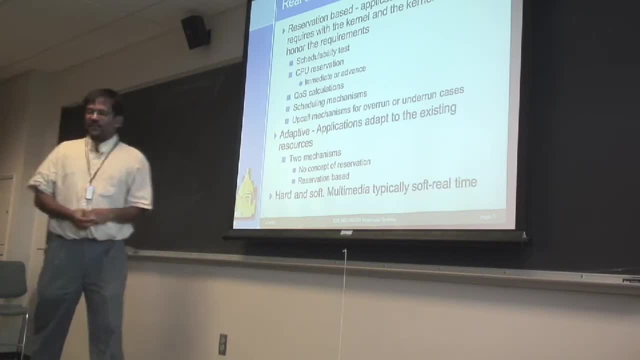 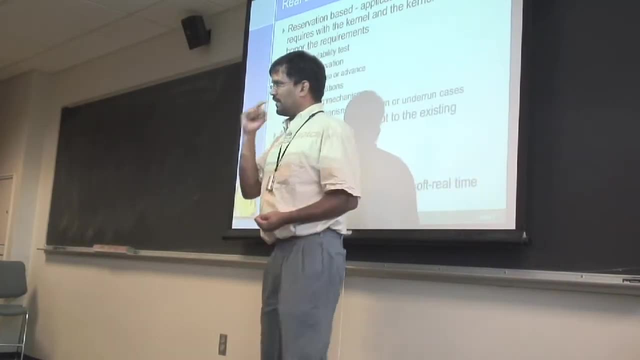 Yeah Yeah, It's kind of easy to figure out what they're trying to do because I think they Vista calls it glitch, free programming right, And I guess that means that it's running at a higher priority, higher real time stuff. 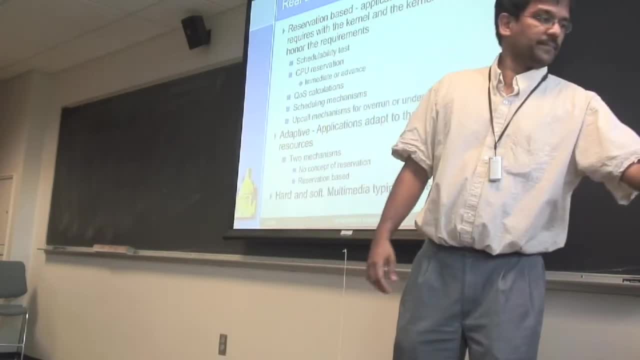 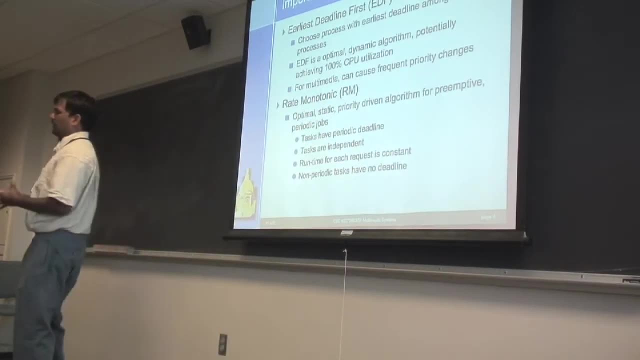 that nothing can cause a glitch for it And sort of the two theoretical or important real time schedulers that you ought to know is the EDF and Great Marathon. Okay, I mean, these are the basic 101 scheduler, real time scheduler, kind of thing. 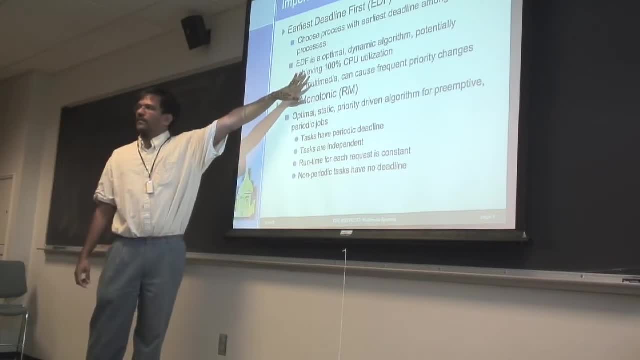 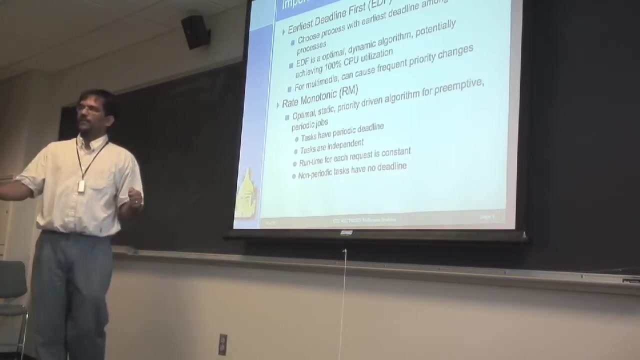 So the fundamental difference is EDF is a dynamic scheduler and Great Marathon is a static scheduler. What this means is like when you have an EDF, it sorts the runnable processes based on the earliest deadline right, So it has a notion of when it has to be run. both of them need a notion of when it has. 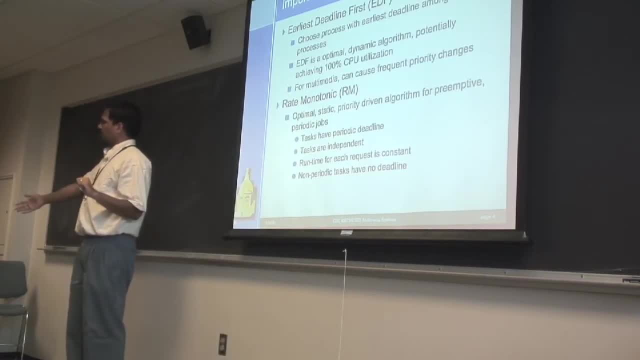 to be done, Okay, Okay. So it's a dynamic scheduler, the surest right And it can prove that it's optimal within that constraint right. It's optimal in terms of using all the CPU resources, So it will miss deadlines. 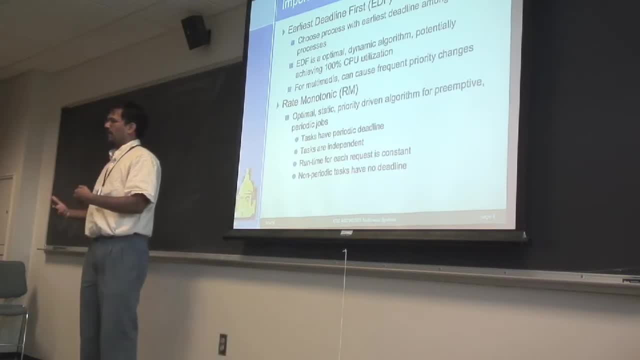 But for a dynamic algorithm where the decisions are made on the fly. it'll give you the optimal decision and it can potentially achieve 100% CPU utilization. Right, You'll miss deadlines because if you come into the system later than when you should have, then you'll lose out. 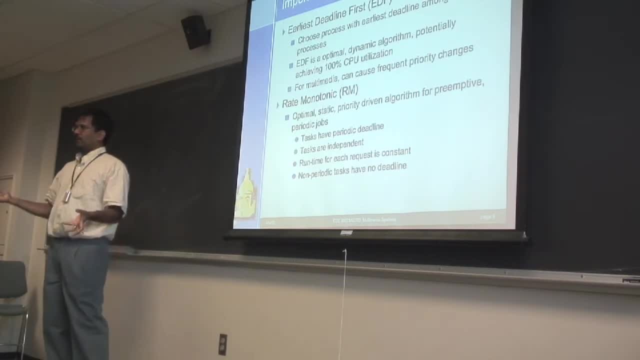 Okay, processes in the system who have higher practice than you, then you don't get to go right. so your notion of priorities which affects this stuff, so within those constraints, that's optimal, right rate, monotonic use. you say everything up front. you say what, what, what you want, what the different priorities are you. 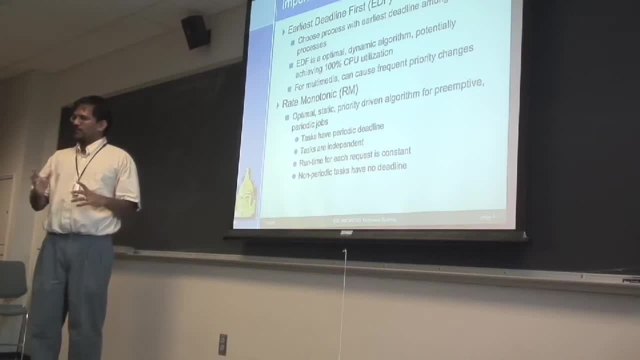 figure out what the schedule is, the schedule and never change. the schedule doesn't change on the fly, right, so you don't miss any schedule because you, upfront, you know what has to run right, the. the key here is you need to know what those, what the but what you really want, and you can't change it on the fly. 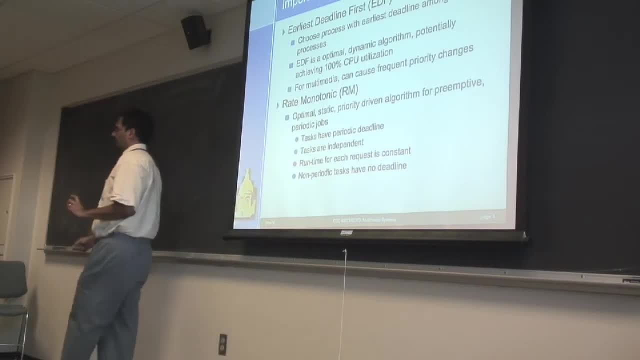 right. so if you say every second I want 10 millisecond of CPU system, can give you 10 millisecond CPU, right. it's good if you, if you only want a 2 millisecond, but if you want a 12, there's no guarantee that you will get that right. 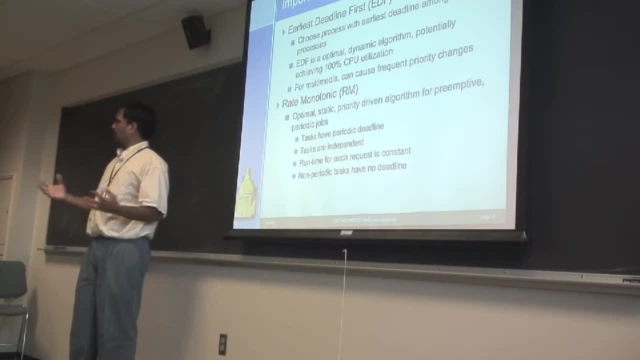 because it's static that nothing, nothing is done afterwards. so if there is some CPU left over, you may get it, but you're not allowed to change it on the fly. so each one of them, you know, have some good properties. mostly they're optimal, but there's some. 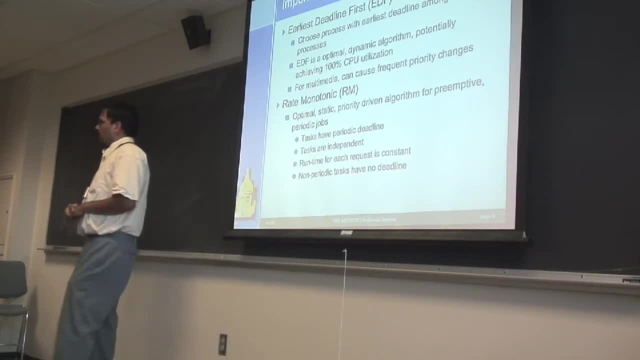 bad properties in in terms of what, what you do for multimedia right. one of the stuff, one of the important things to notice is, when you play with this priority based schemes, you have to make everything that that you're using part of this priority right. so if you're, if you're a browser and it's running at a 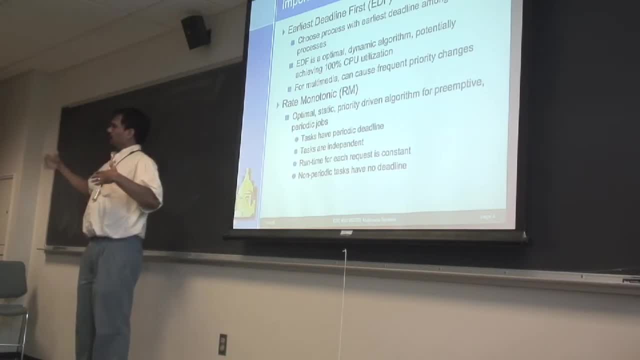 higher priority and it's getting some disk IO, it's getting some network IO, it's getting some memory buffers, it's getting getting some what, whatever in the system. right, they all have to be in the same priority or same pseudo priority, or else these systems don't work right. so if I want from the highest priority in the system, 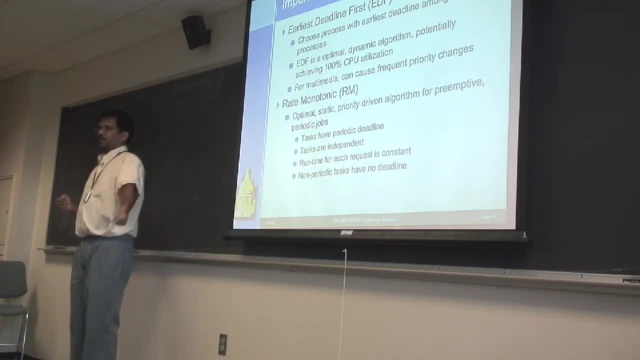 but if the network system is not at the same priority as me, or a proxy is not the same priority as me, right, then I'll basically start, because I get to go, but the I don't get the data in the system enough, right. so if I don't so, if I don't do that, the other other problem. 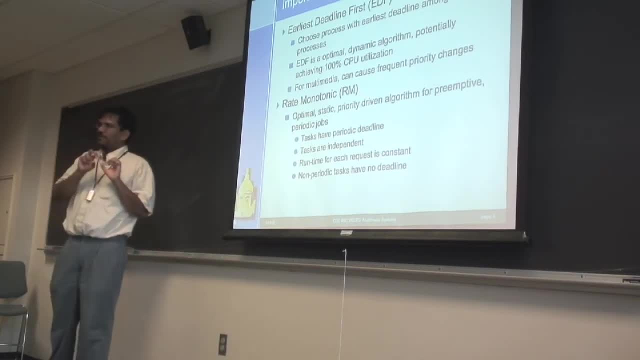 with the priority based schemes are: if you don't have the priorities right, then I may be booted off too often, right? so if I like, for example, if you use the earliest EDF scheduler, right? so anything which is which comes to the higher priority than me would kick me out, right? anything which comes to the with the 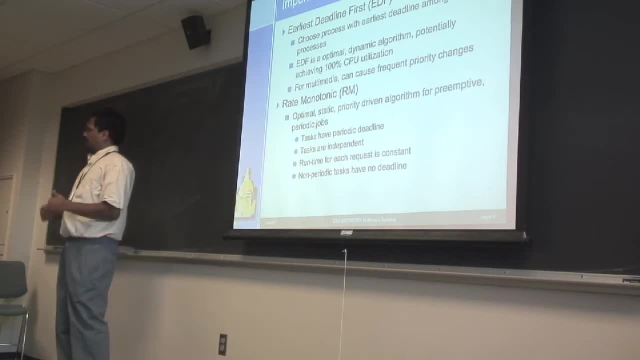 other same priority but the. but the earlier deadline would kick me out and since I don't know upfront what kind of system would be running when, when this whole system is working right, which is more similar to what you would do on a desktop, right? so I may be getting booted out a lot, I may be getting lots of. 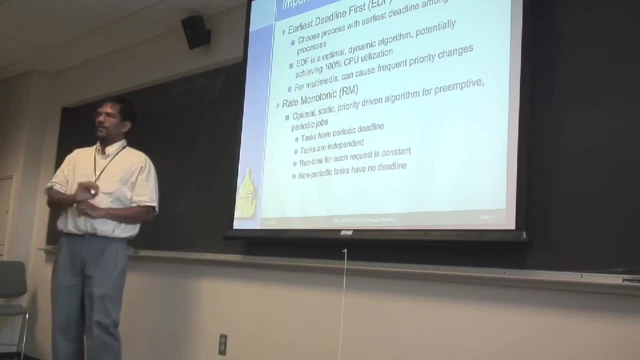 interrupts, which may actually kill my QoS more than you would want, right? so if I only get time to work on half my frame, I may not be able to show any frame at all. so even though I only get half the CPU that I asked for, the screen may just be blank because I don't have time to do anything at all. 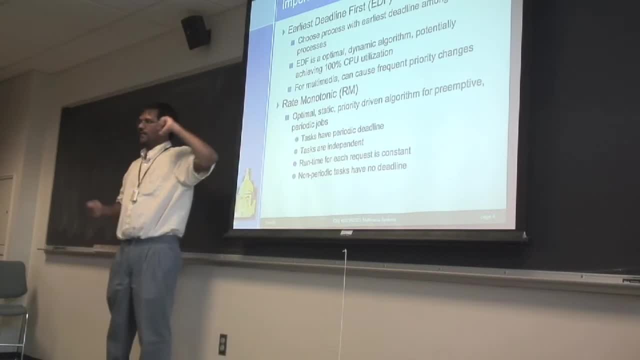 right. so- and those are kind of hard to explain in these systems, because I can't say I need at least this much right, even though I may have lower priority than somebody else, you have to give me at least this much resources so I can give you some quality video. not, you know, rather nothing at all, and so that's. 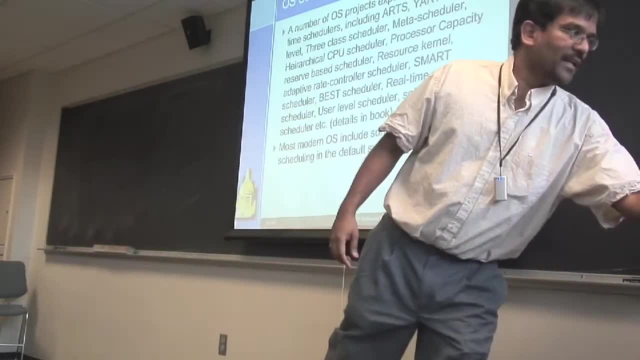 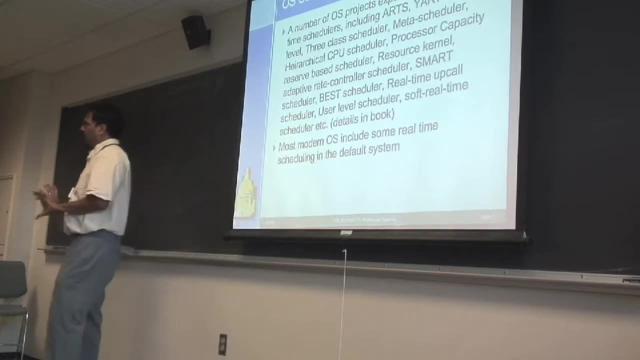 where all the other research projects? I think I'm gonna lay out some of the names and your book goes through some of the examples. right, there are a whole bunch of projects and essentially they were their variations of EDFR or rate monotonic and they're trying to fix these things by using 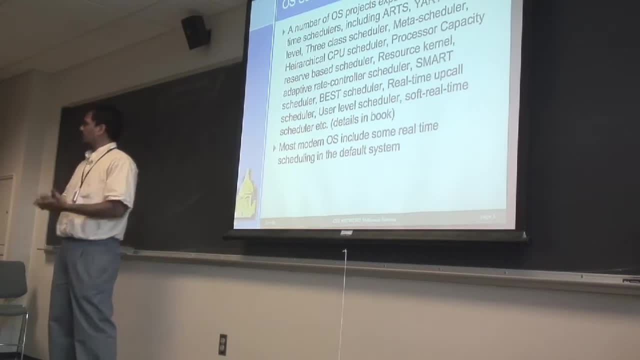 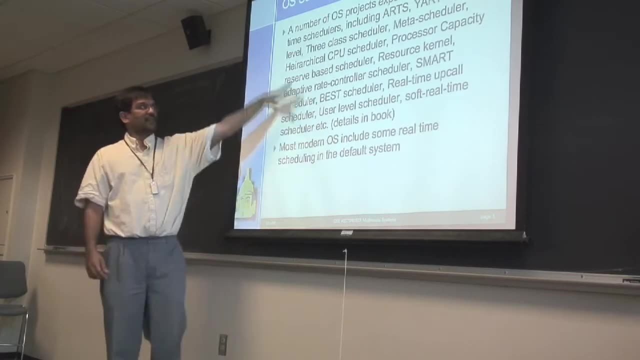 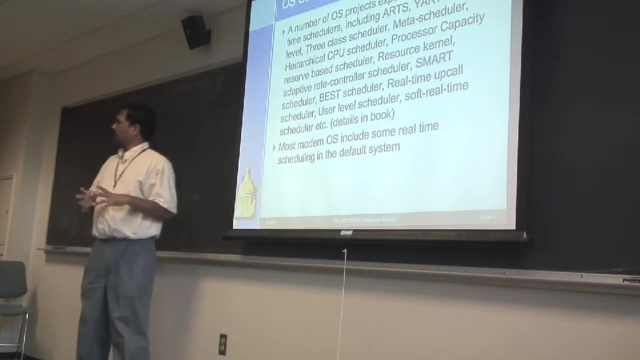 different schemes. so you see, you're trying to make it look good. you know, do a good job for multimedia. it won't be optimal, but these are more practical, right, and the key thing for you to notice is: I think the the latest one was smart. I think that was in 2001, I think, but in terms of the, when they were, 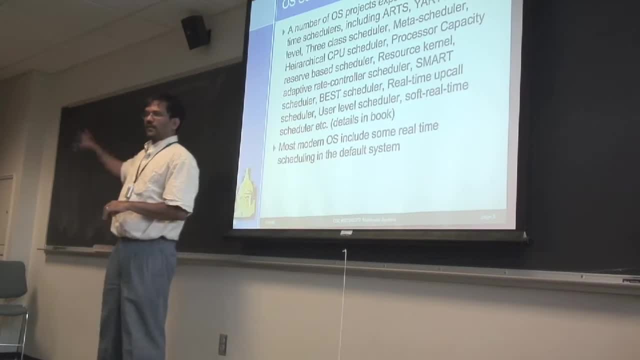 published and stuff. right, many of them are right. many of them are published in late 90s or earlier, right, and we're in mid 2006, so there's been a while when nothing has been done. right, it's exactly not true, but you know most. 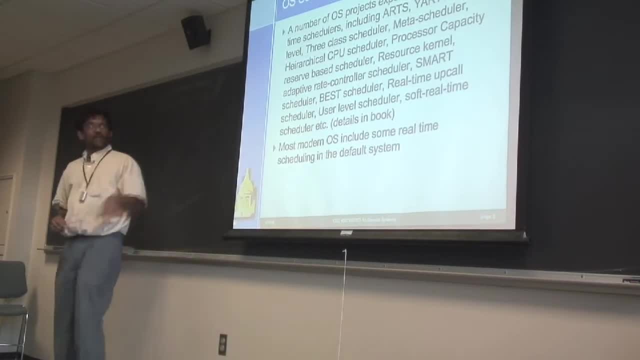 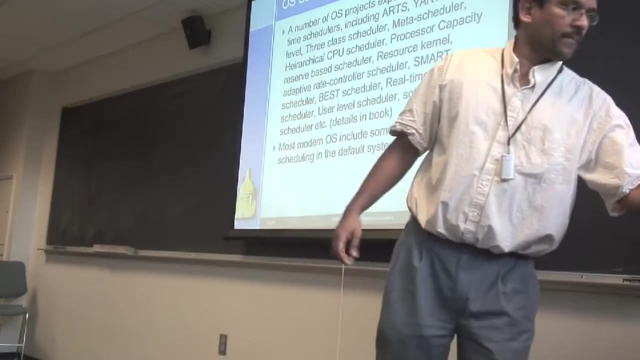 modern operating systems do have real-time scheduling built into them, so they may use a variant of one of these things inside them. we just don't know the exact specifics. so I kind of alluded to the fact that you know CPU is not the only thing you. 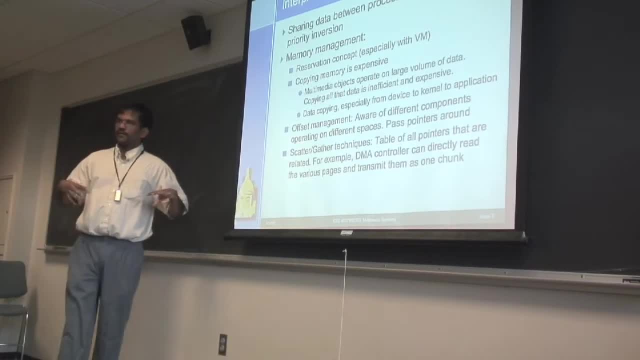 need to get the CPU to work, and you need to get the CPU to work and you need to get the whole system to work, especially if you're using inter-process communication, in whichever form you. you mean that you know whether you are passing messages between applications or for the terms of next slide, in terms of 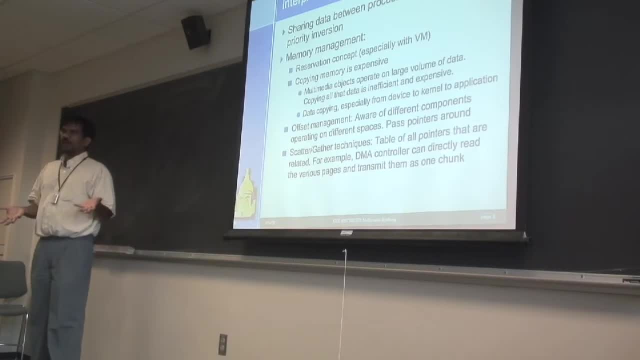 allocating memory. you have to give them the same kind of priority right. your Mac OS X uses mock operating system, which is a micro kernel, but essentially where messages are passed around the system a lot right. so the idea is to have- I'm sure you talked about in the in the OS class, essentially a small kernel which is good at doing. 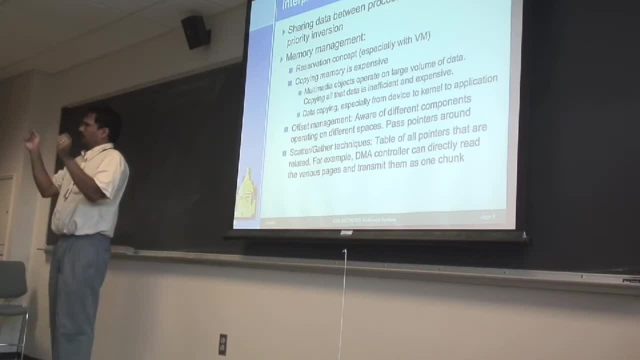 something and everything else is pushed up to the user space and they communicate with each other to get some work done right. so those messages will have to have the same priority as the processors, or else this whole scheme would fall apart, because I have a message I need to send. 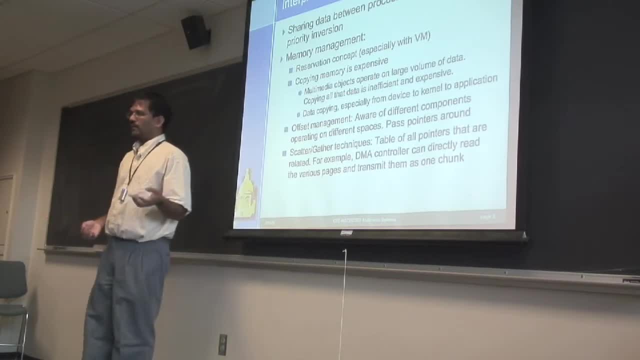 but I can't actually send it because I'm at a lower priority. what have you right? and? and these are not trivial, and these are, these are important things. and then there are various efforts to do that. it's not trivial because some of it, if you look at the like the regular OS, some of the layers may not even have a 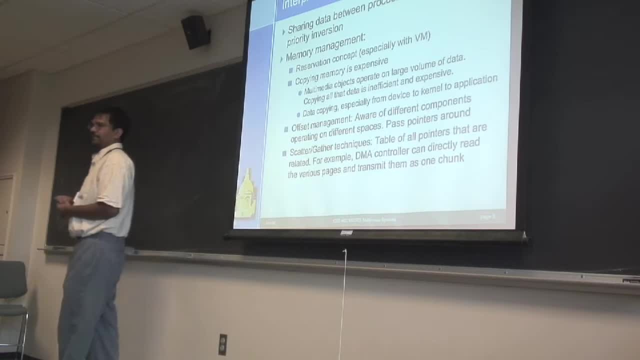 notion of this right, for example, if you get an interrupt, if you get a device interrupt right for, let's say, if this block is it's read, it's finished, or this block is ready to be read for you to do something. right, if you do this, this the different priority level, right. I may say that this 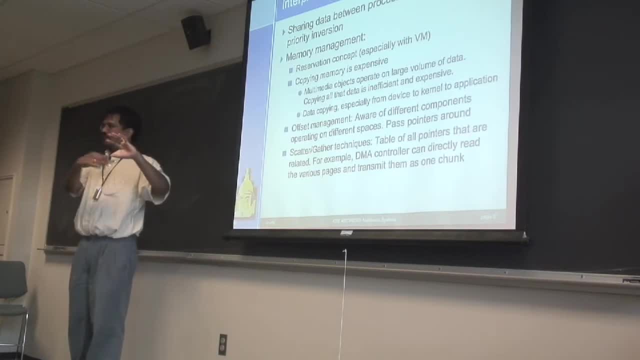 layer requires a lot of disk IO, so so have it read fast, right? if I get an interrupt from somebody else that I know it's not the higher priority, I I don't want to accept it. I just want to say: go away, come back later, right. but the problem is I don't know who's coming from, because I need to actually 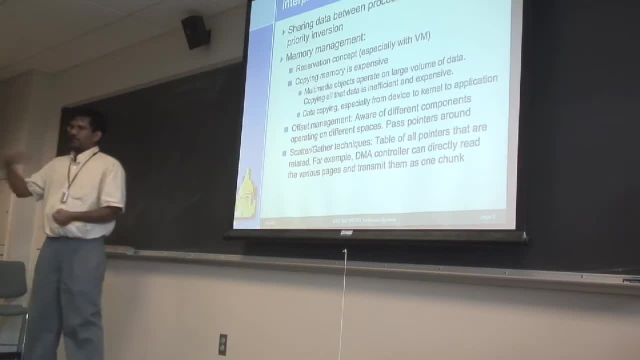 process: the, the interrupt. I need to open the interrupt I need to figure out. read some of the bytes in to figure out that it's not for the higher priority process. so I gotta throw it right. it's especially true for network process. right if I do. if I get a network packet I I may not want it, but I have to do something to. 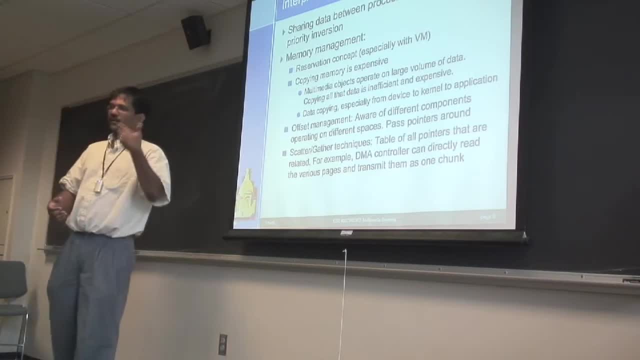 know that I don't want it. I need to read it, get it up the kernel stack to some level and then open it, read it and then find that it's not something I wanted. I need to throw it out and that by that time you you're. 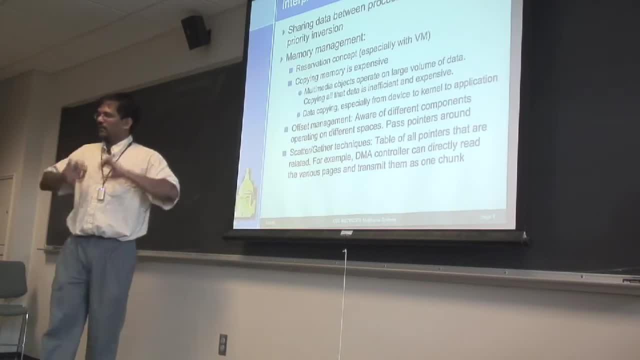 done a lot of the lot of the work right. so moving this into the, into the stack, it's not that trivial. it's not just figuring out associating priorities to different packets, because by the time you can associate it's already probably too late. and then there are some work, work in trying to to, to solve, solve these, um solve, solve the notion. 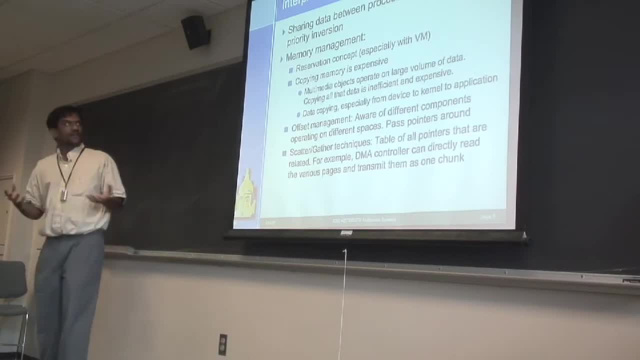 of of inter-process communication stuff. the other other thing you want to worry about is memory, because that's, that's that's the, the four of the things that operations manage. one is a CPU, another one is inter-process communication, the other one is memory, the other one is the. 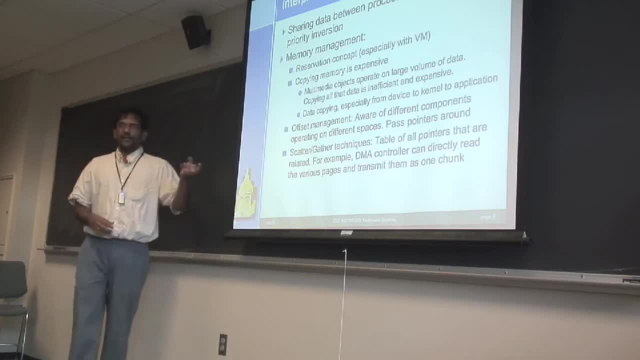 system, which we'll look at in a separate lecture. so here the idea is: you want to have the, the media, the media applications have enough buffer so they can make progress. right, if you're running on a virtual machine based of system, if you keep stealing all the packets from these process. 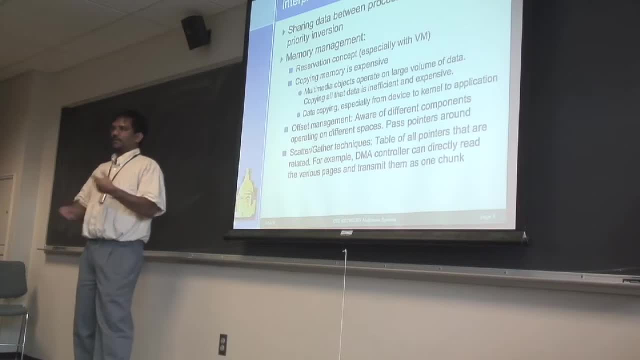 essentially every time you the process starts to run, you'll have to do a page fault and get these stuff. so it needs to be able to, you know, pin down some of the pages in memory so they won't be swapped out and again you need to worry about. 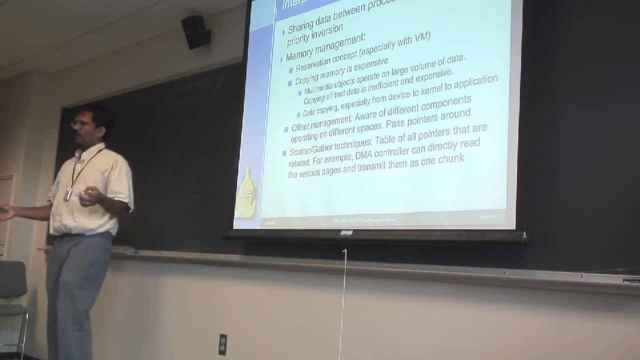 how would you do this fairly when you have other applications, right? so if you have, if you only have, 128 megabytes of memory, how do you make sure that this video application, which needs 96 meg, would get that and still be able to do something else? right? how do you, how do you make, make sure that? 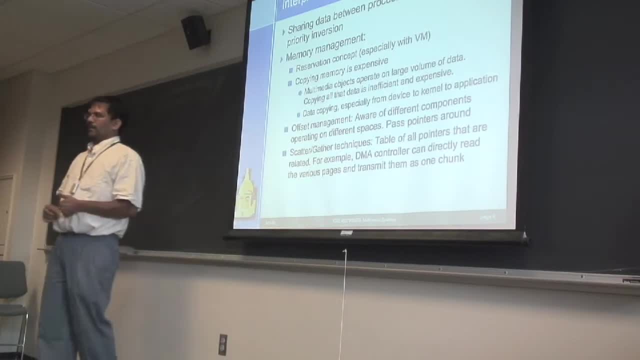 there's that these are pinned down. that's one thing you need to worry about. the other thing you need to worry about is memory. copy operations are very slow and you try to optimize around those in in in. in general, multimedia operations tend to move lots of data, so any inefficiencies you notice there would affect you. so you need to so many of the 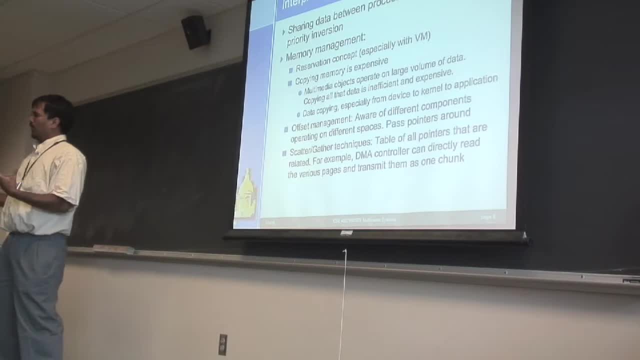 techniques that you develop, are you learnt in OS for avoiding copies directly are applicable to multimedia objects, because you're moving lots of data from the disk or what have you and some of the mechanisms that you may or may not have looked into in the, in the, in the OS class, depending on the on the level, are ways to avoid these copies right? 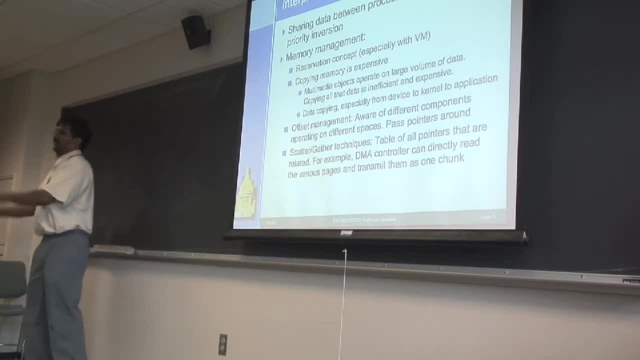 so the simplest way to do that is you. you read it from the device driver into the kernel, you read it from the device, from the kernel to the user space, and so on. one way to do that is to deal with his using pointers, right? so rather than copying this stuff using pointer, so your 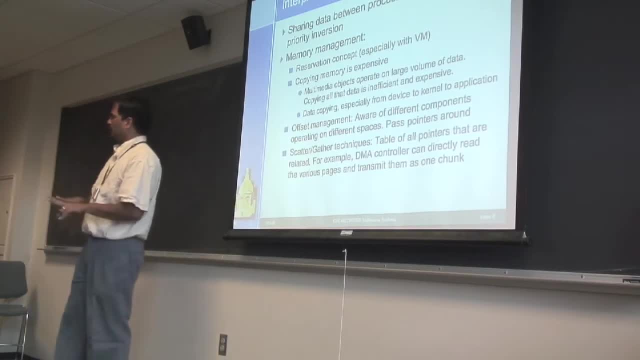 your system should be aware of dealing with stuff in pointer. so if I, when I read a chunk of data, it may not actually be where I thought it, it would be right. so if I say, read me a buffer, it may be an address that is more suited for the system rather than into a variable that I want right, so be able. 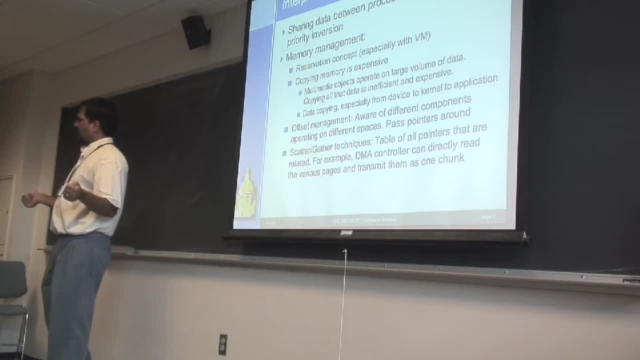 to deal with those or be able to do scatter, gather right, which I think in the OS I mentioned- maybe a word of it, but the idea here is, if you're doing a DMA or something right, rather than saying I want you to send this big file or this big memory out to out to disk. 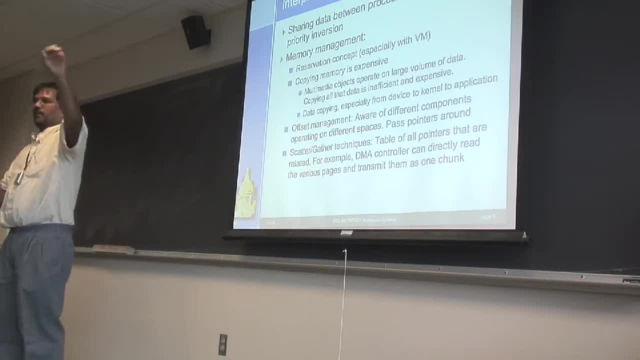 being able to say: this object is, you know, part here, part there, part here, part here. the header is here, the contents is here, the trailer is here. collect everything and send it off, right, but wait till the last moment. so you essentially have all these things floating all over the place. 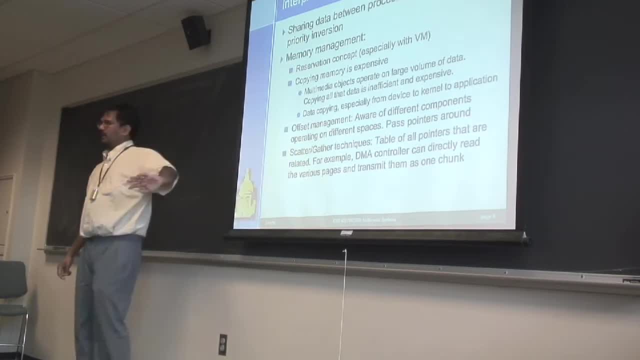 right, and these are not techniques that are that are designed that that that you, these are techniques that you have studied in the OS class, but but the, the motivation for those usually come from multimedia right. so I'm kind of on the. to me, most of the, at least the desktop operating systems, 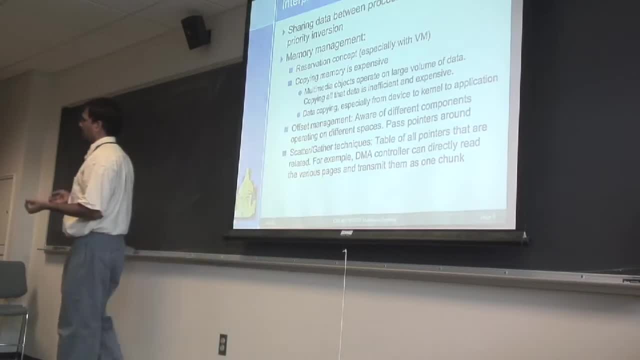 any development you see is basically because of multimedia, right, because they kill those machines. they're the ones which may require all this stuff. so any of the advantages you see from these on the OS side was probably motivated by by one of these things, because there's a lot of data to move, right. 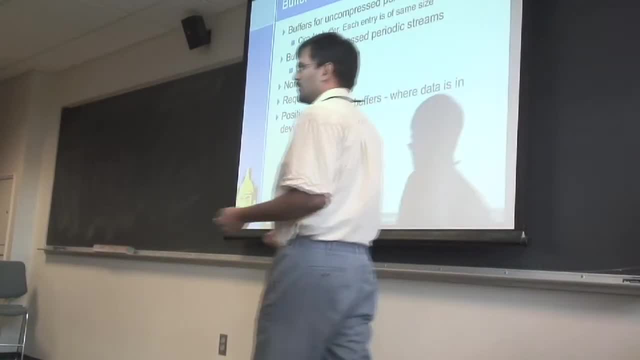 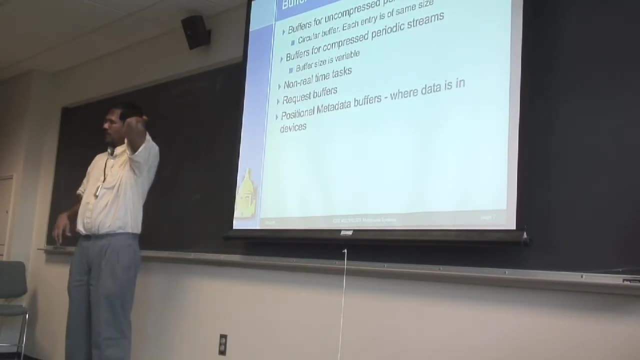 I actually think that if there's no multimedia, we'll still be with Windows 2000 or whatever. right, because Windows 2000 can do most of the stuff that we would want. but we want aqua and all those cool things because they are, they are good to look at, right, and they they expose us to to read some of. 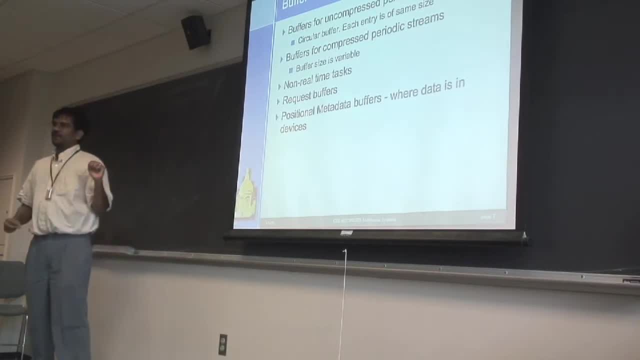 this stuff right in terms of buffer management, the the issue here is: how much? how do you manage buffer if you're giving it on demand to different applications? some of these media applications may suffer because they want lots of buffers, right, they don't want to give up the buffer because they they know that they're going. 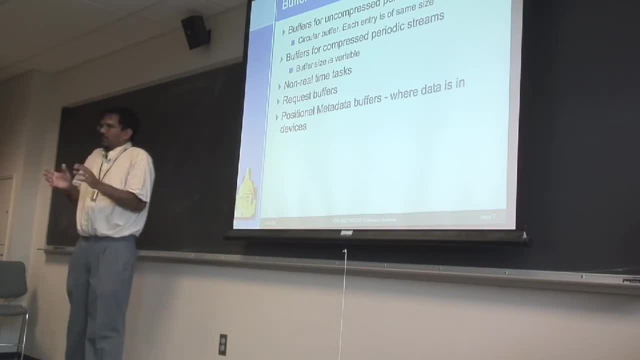 to get an x frame in some some time, so they have to be given some buffers. you can't just take the buffer away from them because then they'll perform poorly, right? so if you're doing HD, HD level video, and you only have memory up to you know, say, half of the frames, then you're constantly thrashing. 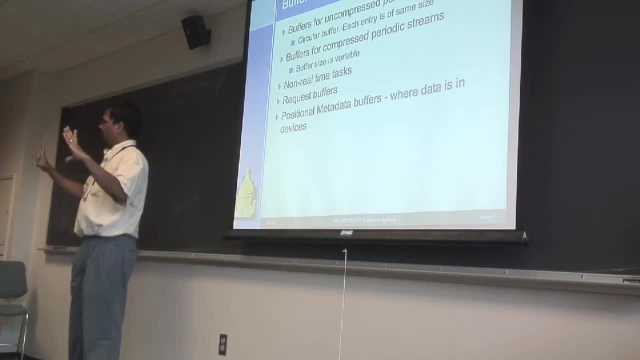 because you know, as an application, that you need 1920 by 1080 worth of buffers. but if you can't hold on to it and if you're essentially asking on the fly, then you're going to suffer performance. performance, wise, right. so so being able to reserve buffers, being able to, like, pin them down, and and all those things, 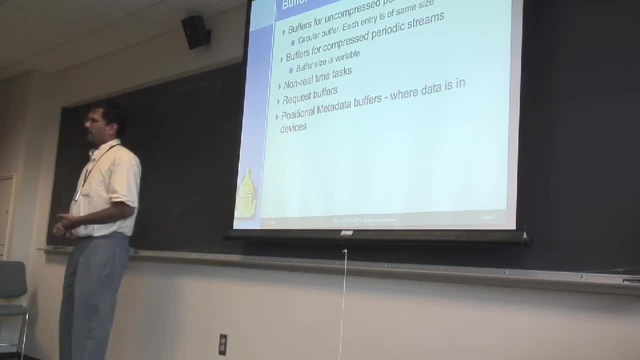 apply through to the multimedia streams. right, the question is, all these are trivial. the the harder part is: how do you, as application, express them to the operating system and how does the operating system figure out whether you can be trusted? right, if I export this to a regular user, I can't see why anybody would write a program which 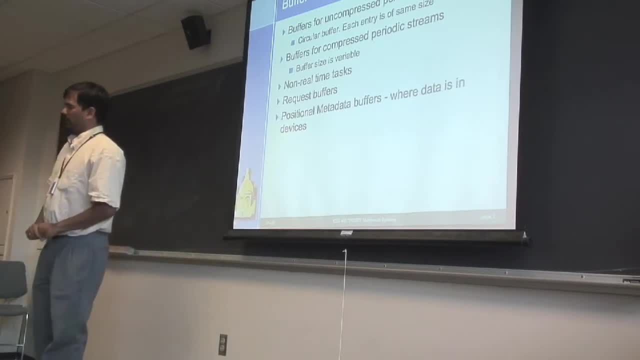 says: I'm going to play nice, I'm going to give away all my memory. right, you would want to use some of these facilities to say: any memory that I get, I want to hold on to it because my application will run faster, right, and that's, that's the harder part than being able to implement this within the within. 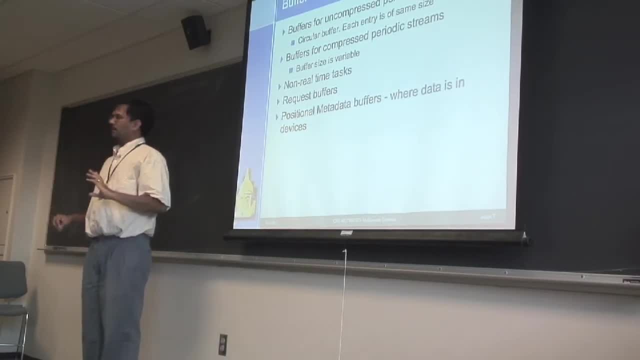 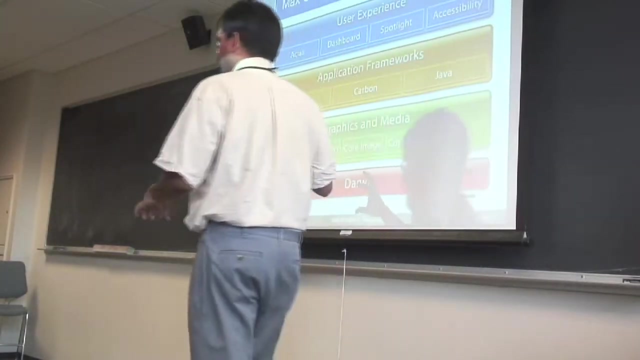 kernel. right being within the kernel, you can say the mechanism to implement this is trivial, but the policy of who should get them, who should be able to specify them, are the hardest part, harder, harder. so I'm going to kind of jump into what like what, what your Mac does I was able to get. 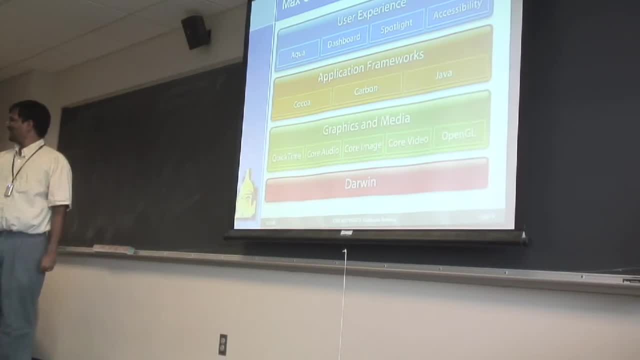 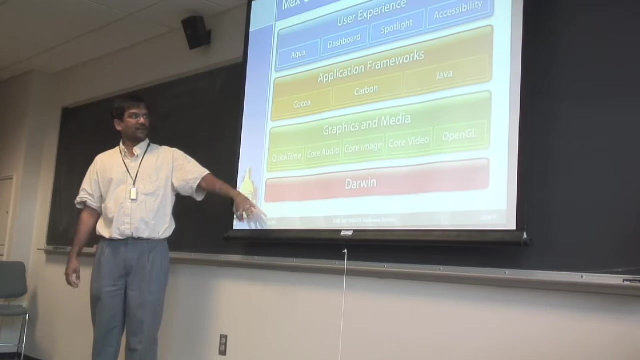 a cool video out of this one. really one thing, right, this is the only video that they had which actually looked cool. I think somebody mentioned there's no graphics in it in a while, right? so essentially, this is your operating system, right? this is your, your kernel mark, kernel running, but from a user perspective, these are all the stuff that you see that there's. 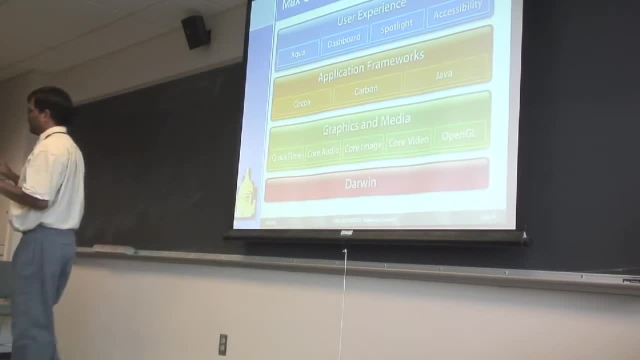 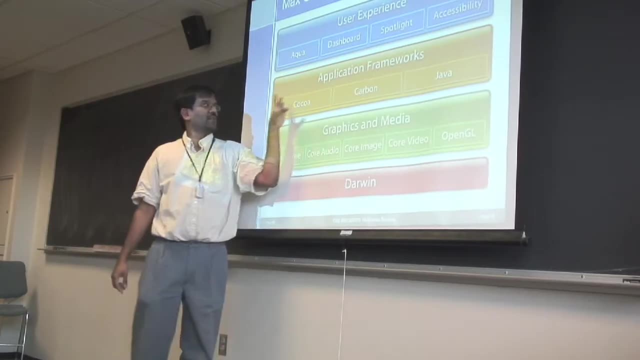 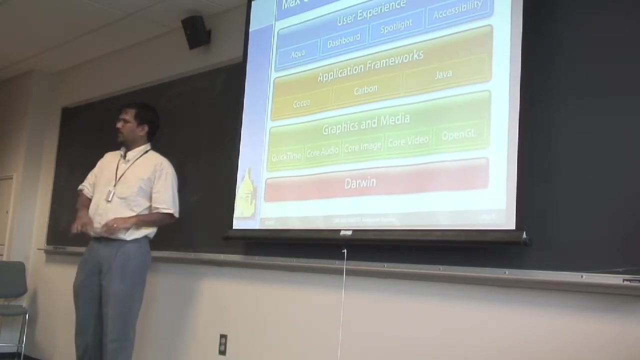 the, your user experience. you know the, the aqua interface with the buttons and all those things. and then the application development framework: you know. now it goes to the version of Lllo or Karbon or Java based right and and, and windows has a similar notions of. 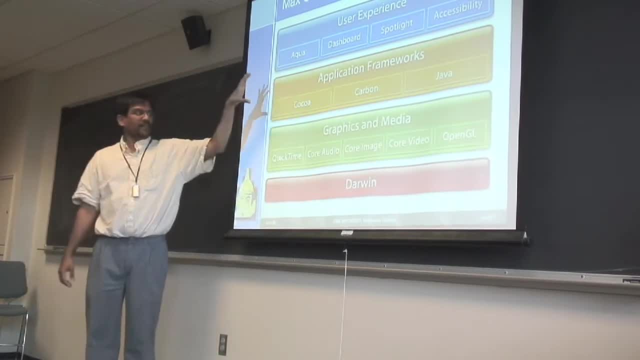 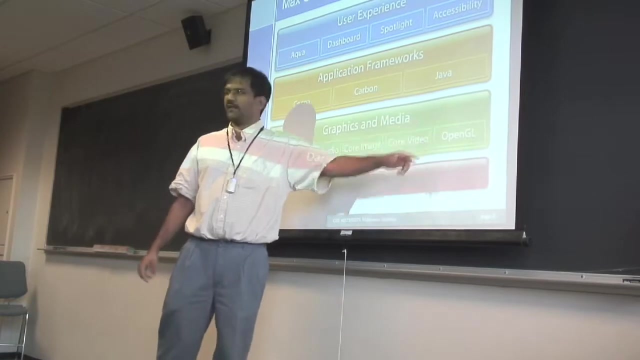 servedgesch and for for Mac, the quicktime library is pretty powerful and useful. there is also the core audio image video for the next version they have. some have the whole animation right. essentially, these these all form a local video right and you can activate that in the per 2015 CPU video. that a truly needs right anyway. sometimes in Intel applications it's made so that, for example, if you enable Windows x, uncom لا تُ༠ه sub مركز Hiόło anos starts siliconean and use windows in that. as you can see in Windows x, Windows is not exclusive. 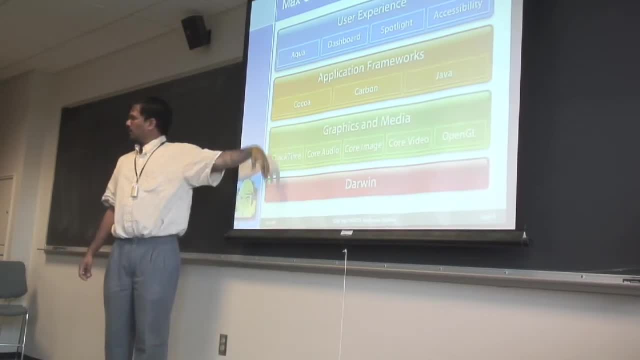 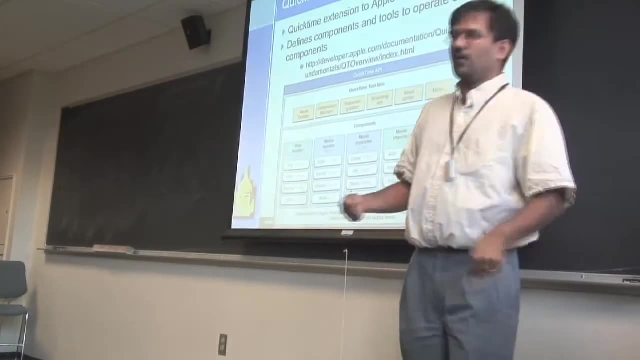 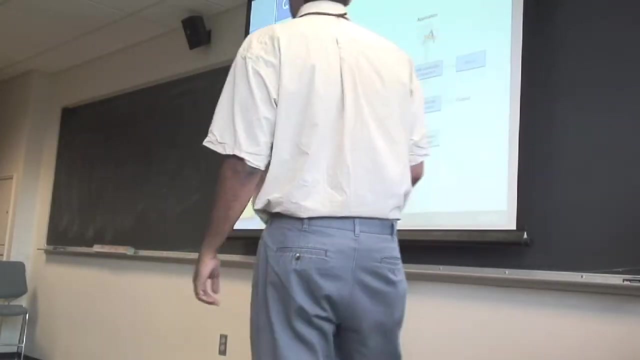 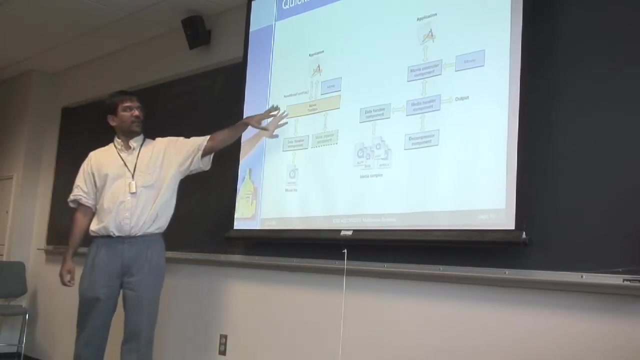 layer so, and they interact with the, with the, with the kernel right, and they can implement certain policies. so the idea here is: if you were to develop a code to capture videos or frames or what have you actually? it's the, it's one more side over. if you use the quick time component right, essentially you can you. 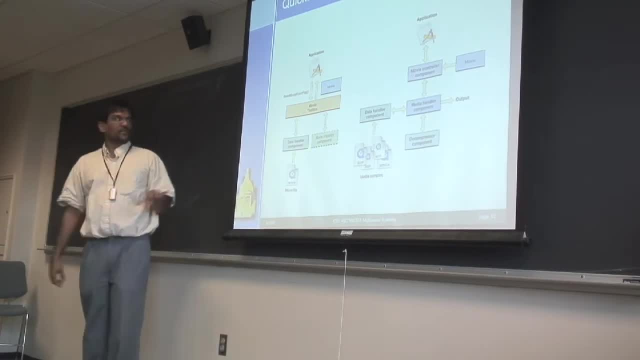 can build using these different components and operations on those components. so to read a multimedia file, right, so you would call the movie file. you set up the right data handler to read either from a file or from a network connection, right, and the movie tool box gives you operations like play. 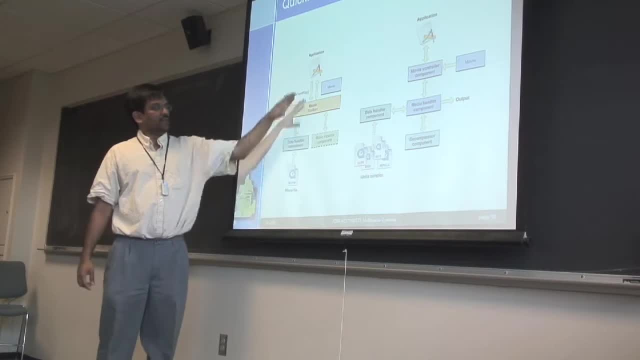 or what have you right? so in this case you can read the file by defining this movie object, defining where the input should be, and then do the read operation and then it will figure out how it should be. you read right, so they can move a lot of the functionality in here to do some of the 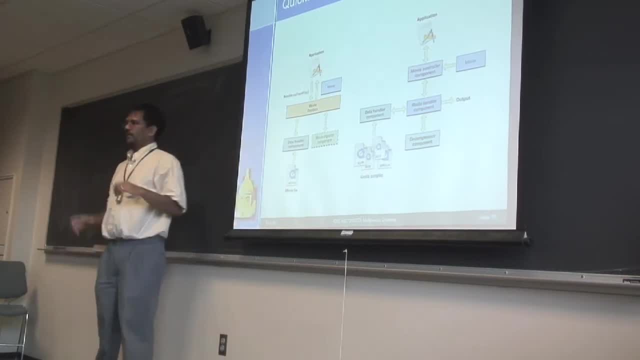 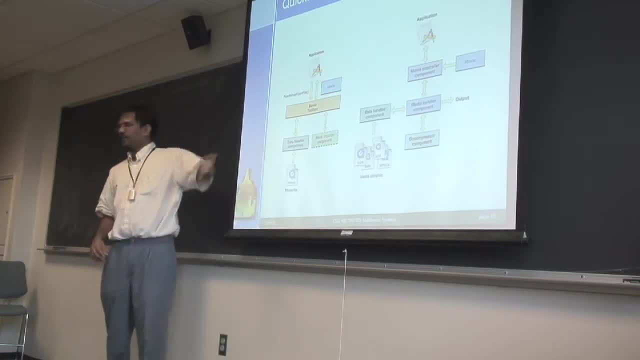 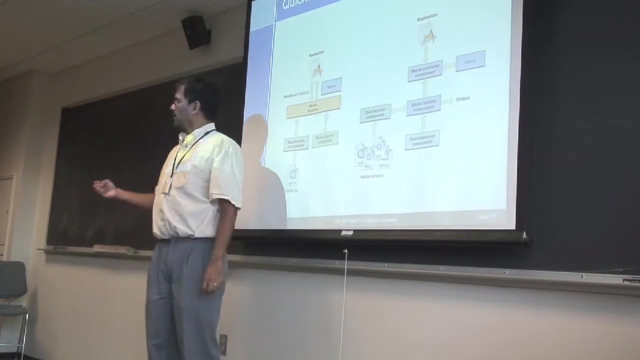 inside the kernel- right, it's not kernel, but it's. it's something inside the pseudo OS that when you use this stuff, you can actually get a lot more of these things. and this is, this is how you would. you would do how you would view this movie, right? so 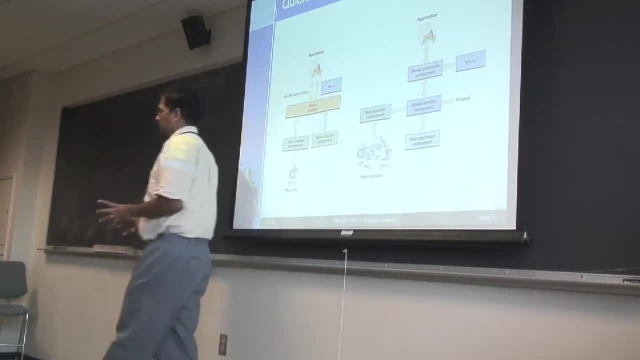 call the appropriate decompressor component, depending on how it was compressed. so you say, open this movie and then play, and it figures out what other the decompressor it has to do, what are the transaction has to do, and then and then play for it, right? so if any of you have to want to develop any kind of code for 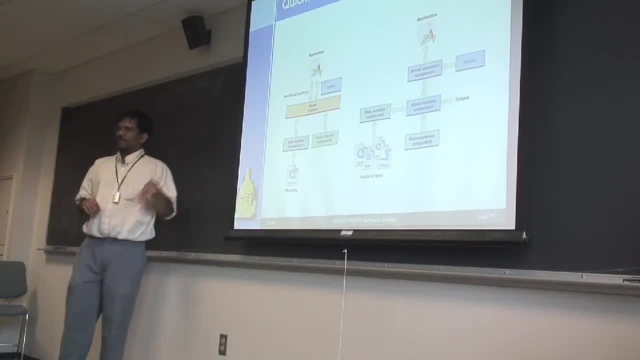 your course project or something doing video right. I suggest you look into the quick time the, the programming component, because it's very easy. for example, if you, if you're ready from Firewire, you don't have to worry about the Firewire issues of how to read and all those things you can say. I want to grab a. 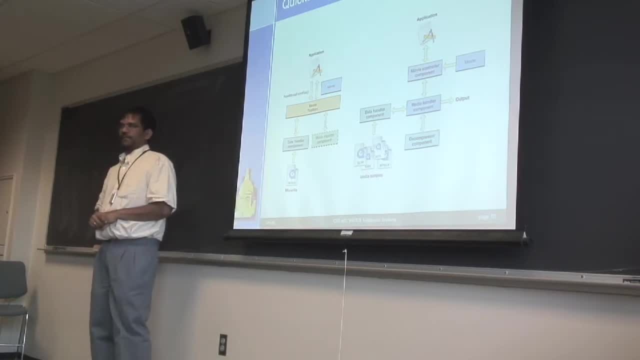 frame and quick time takes kind of a whole bunch of stuff right, but by the same token it can actually do a whole bunch of other stuff. so essentially, if you're on a Mac- unless you you go off and write your own decoder and don't use this framework right, all the all the systems essentially use only one. 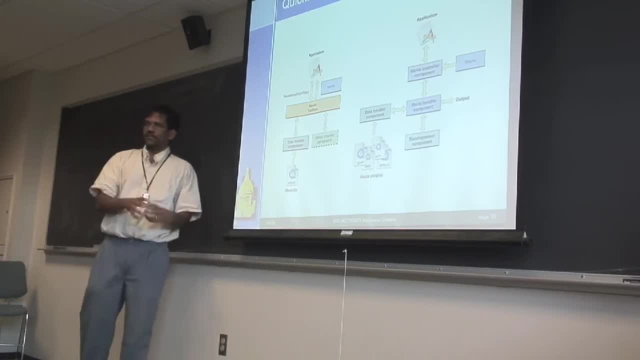 decompressor, one decompressor, one compressor and so on. it's sort of the thing. so if you go to the finder and you see this little movie and you play it, that's using the same component as if you're doing quick time movie player or if you're going embedded somewhere. they're all the same and part of being 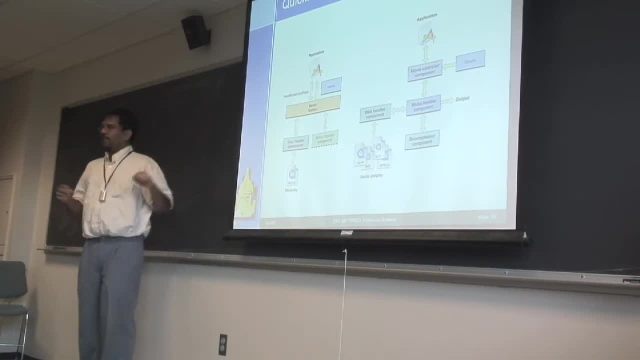 the same, other than like reducing the amount of code, is to be able to make all those reservations and all those things possible if they so choose right. I couldn't find too much information of whether they actually do and how they how they actually do it, but they could. 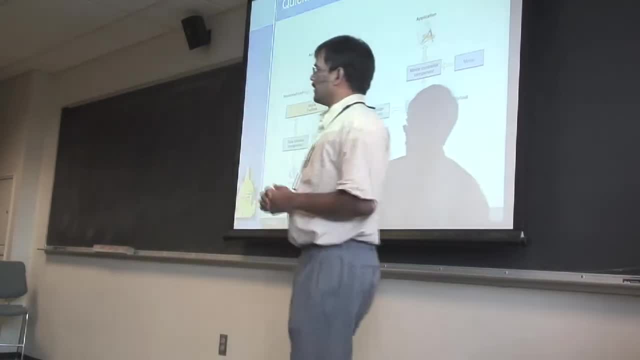 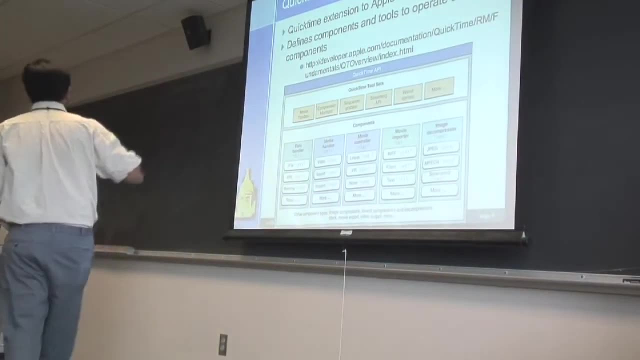 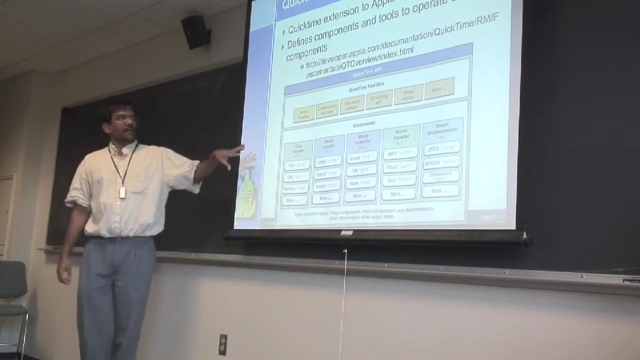 if they wanted right, and you won't be any wiser. you'll just look good to you. so I'm going back to the previous slide. so essentially, the quick time extension is: is the for the Mac OS X, is the? it's a component which, which is used for, so it. 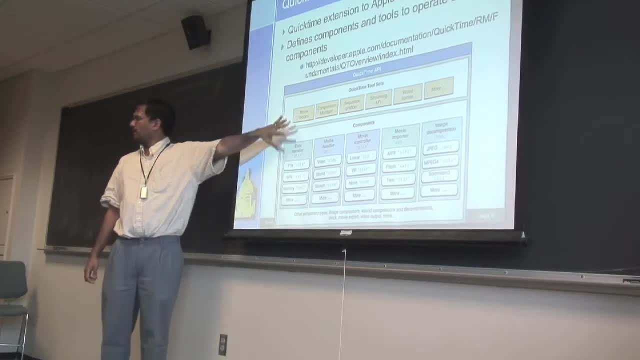 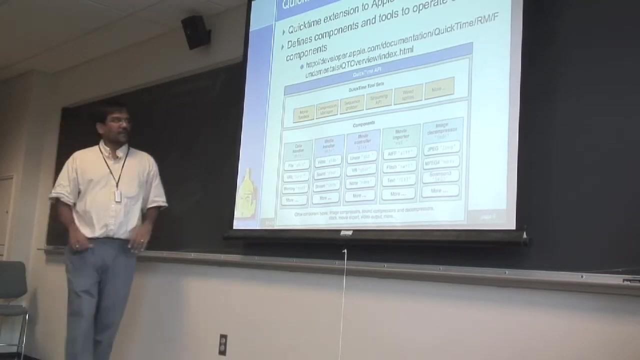 has a set of components and tool set, right. so components are, you can think of them as different kinds of objects and tools or operations you can do on them. so you know, this is the. this is a component I saw from the Apple website. so, for example, for each of the, for the movie movies, you can say that play them. 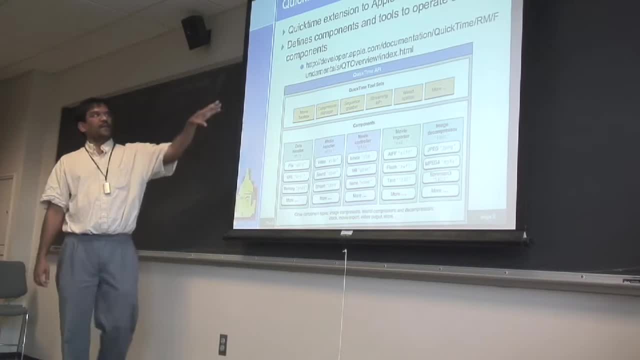 or you know, stream them or what. what have you? and that's what essentially Mac gives you. That's the reason why it's different from, say, running on top of Mac, because you have these, these application libraries which abstract a whole bunch of stuff right. so there's the software engineering component, which 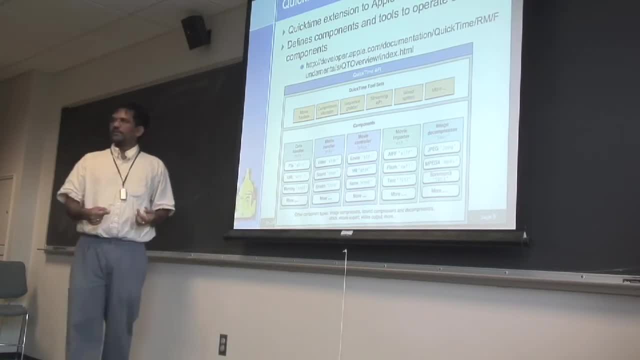 makes it easy for you to code the other component that we are we are interested in is, since it's being done by Apple, into the kernel. they can do many of these operations that may have the real-time systems without even you knowing about it, and, and that, I think, is the potentially the most important. 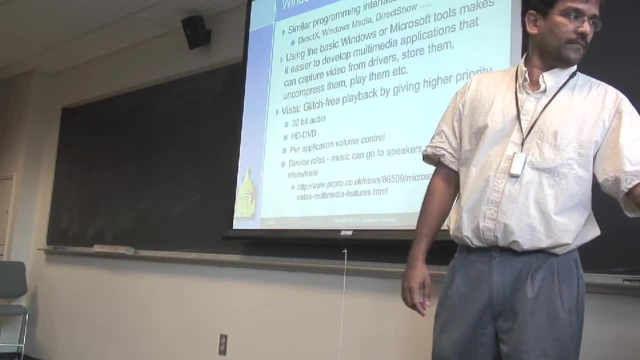 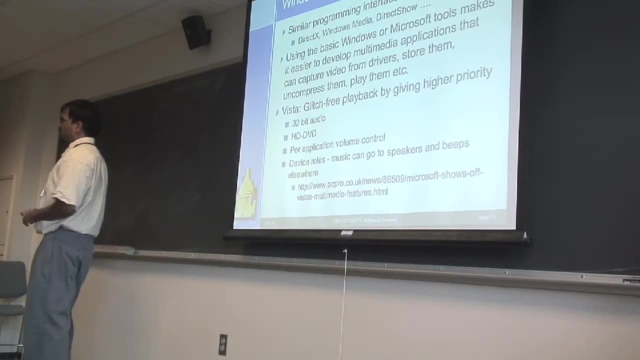 component aspect, and it's not just you know, obviously it's not just Mac, and the Windows does the same. except I couldn't find too much information about it at all, and on the Microsoft site I was trying to see if they have some pretty graphics or whatever. but they, they, they. they hid it pretty well and that's how. 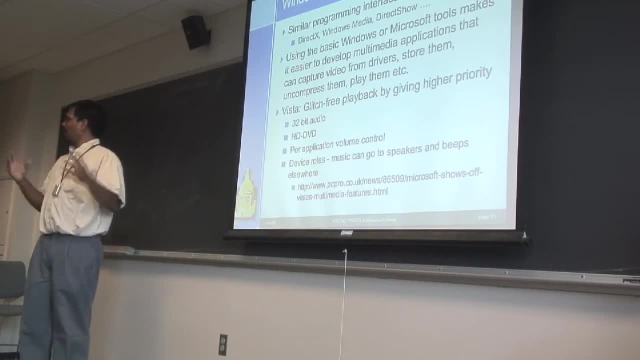 one reviewer somewhere. I don't know much about Windows programming to begin with, so you know probably if you search for it, we were to find it, but they were talking about some of the differences that you will see in in in Vesta right. one other thing: they 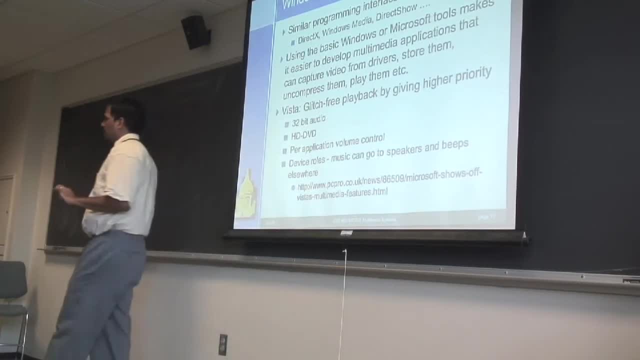 talk about is the glitch free playback. I'm guessing glitch free playback means that somehow it does they. oh, you know it moves you in a different category. right, you know that there's the Windows itself can support real-time and non real-time applications. but since it knows it's a component, it, since it's not the audio, it. 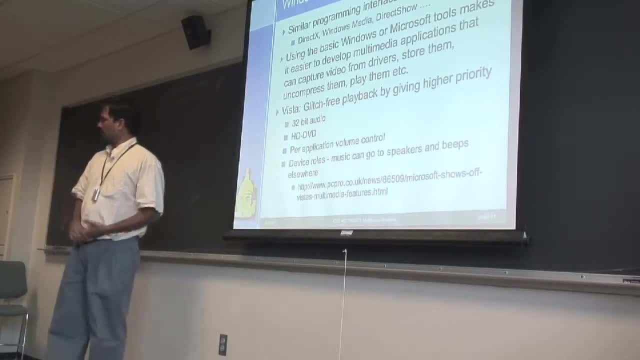 can. it can put it in a different category. it can put it in a different schedule, without you knowing about it explicitly. yeah, it will do 32 bit audio, which is more better quality than you would ever want, right? yes, why, how or what would cause the audio track to be faster, slower than the video track? 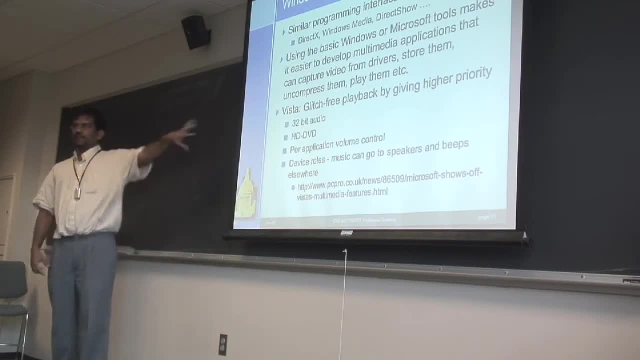 I do know in general, general, right, yeah, if you treat them separately, if you treat them as separate entities, right? so, for example, if you so, the question was: you know why would they go out of sync, right? so suppose you have a video, let's say this is the camera, and suppose this: 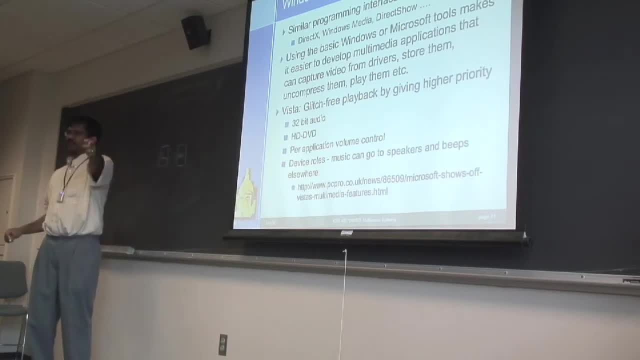 is the microphone right, in sort of in in this model, right, and there's a CPU here and then let's say this is a browser and then capture, right. so the timing aspects of all the stuff is depending on how these, how independent these are, you'll run into synchronization. 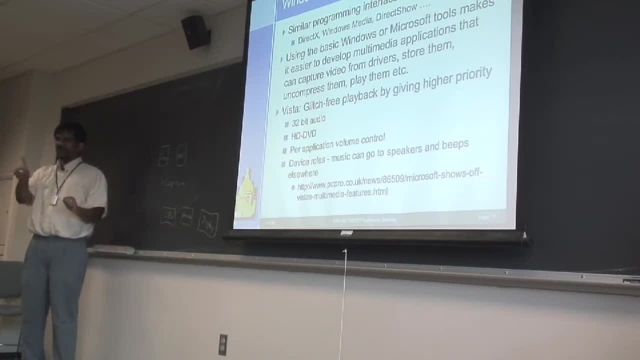 problems, depending on how similar they are. you learn it. to let me finish the thing right. so let's assume this is running its own clock. it's running its own clock, right, if they're both synchronized. if you kind of join together and send it in one stream, they can timestamp them together. 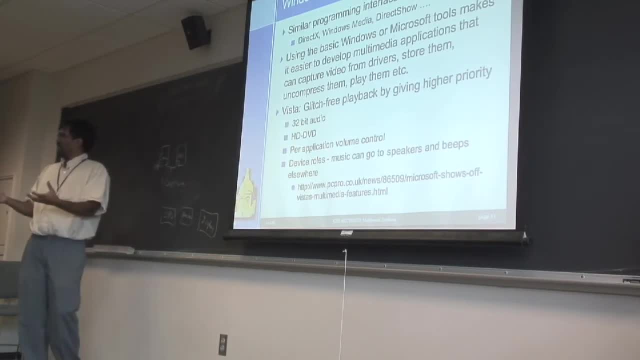 so they are always in synchronization. so, for example, if you use a firewall, right, you, you essentially have the, the synchronization, because your camera kind of puts them both together, like, for example, right now the that camcorder is taking this audio, putting it together and recording it into synchronized form, right, but if your PC, you had the camera coming from. 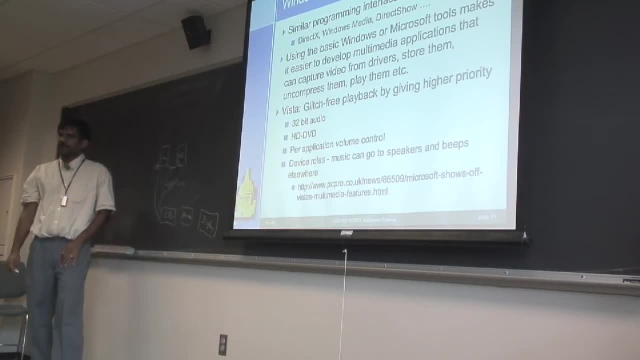 one input and this coming through the sound sound card, right, right. Then somebody has to do this synchronization, right? so because right now this will say: on time, you know? t I caught this frame and this will say I'm I on time, t I got this frame right and in. 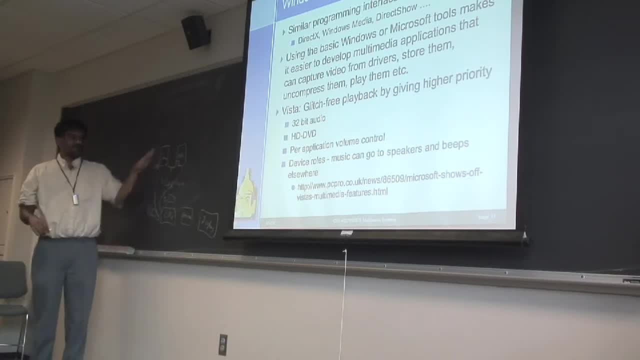 an OS course, at least in a graduate level. you are know that this cannot be synchronized right, because they are the right ποιets, right, you can only synchronized based on what you can see. so you can't really trust these times, you can't really synchronize them. but even if you, 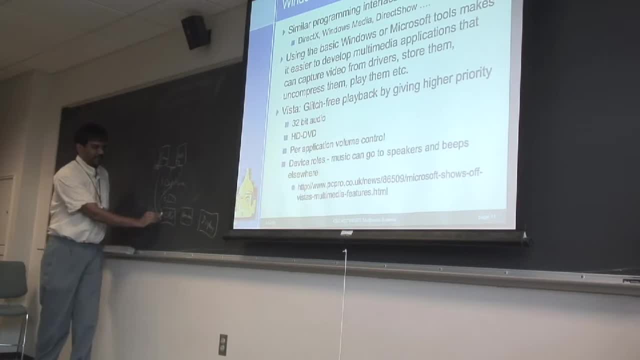 could take those into consideration. something up here: your process has to read both of them simultaneously and and try to keep them synchronized right. if you have two different processors, then it's reading a sound card at a certain rate, getting some packets with a timestamp. then it's getting a video from 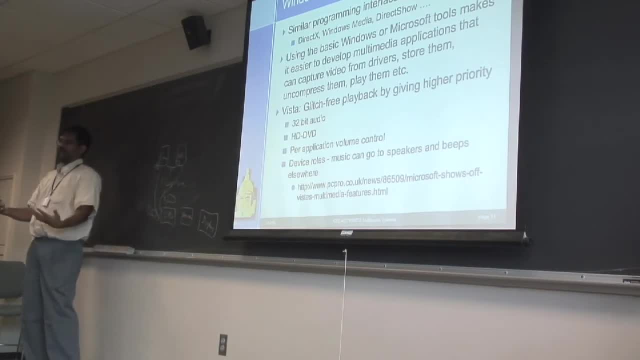 a different thing. it has to time synchronize them, right? I think you cannot. you cannot really time synchronize, but you can make it look good, but you have to make it look good forever. so every frame you get, you have to get this one, you have to get this one. so if you are building a real-time, 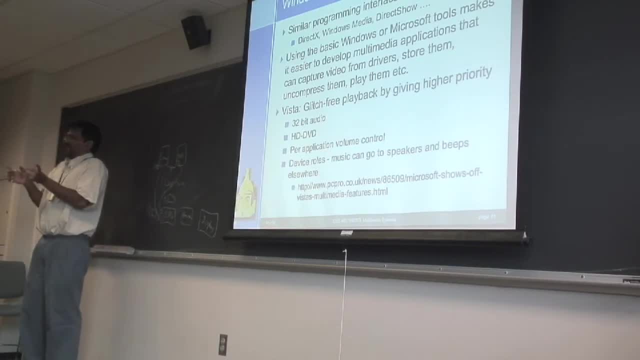 system here. that's two different processes. they both have to be exactly rightly prioritized. where they get this frame, they get the other frame, mix them, send it off. and real machines, real workstations, are horrible at this because you know you're not building a hard, real-time system. 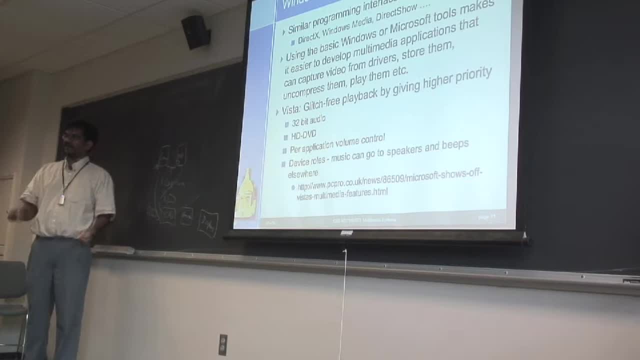 so if you miss something, if you miss your time slot, then if you miss one video frame, right, then essentially your audio would be ahead of the video. so so, on right does that well? yeah, but I also was wondering how that happens with videos that are already recorded with the video and sound are so nice, and then 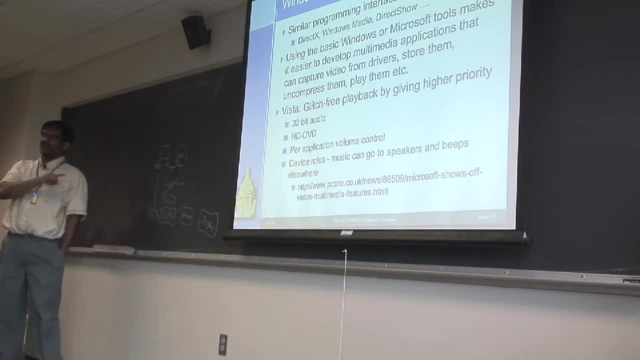 they can, they compress them or something. so within the camera it does a lot of the synchronization to begin with, right? so if you're, if you're, if you have a cheap camera, you, you, you may actually notice it within the camera itself, right, if you bought a camera within the last few, I mean most of the commercial- 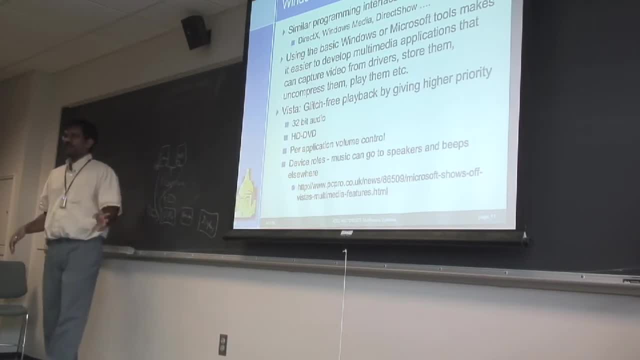 cameras that you can buy right now are pretty good, right. but if you bought a camera like a few years back, you actually would noticeably notice that the difference- right, and so the camera itself may be bad. that it's not synchronizing properly- right, but if it does synchronize properly, then if it's. 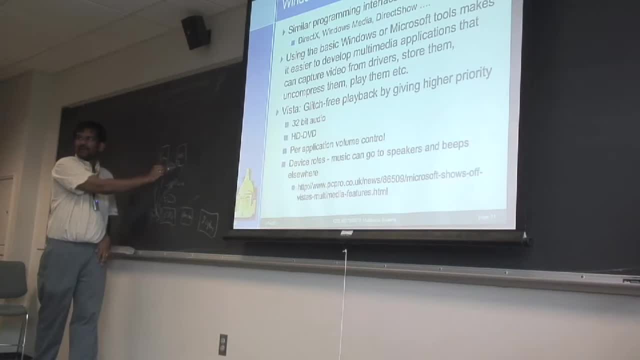 going through a system that's not synchronizing properly, then it's going to single path here, because it does synchronize at this part, then you shouldn't have too much trouble. well, because I just noticed like on YouTube there's some videos where, like, the audio is a second or two behind. so YouTube is 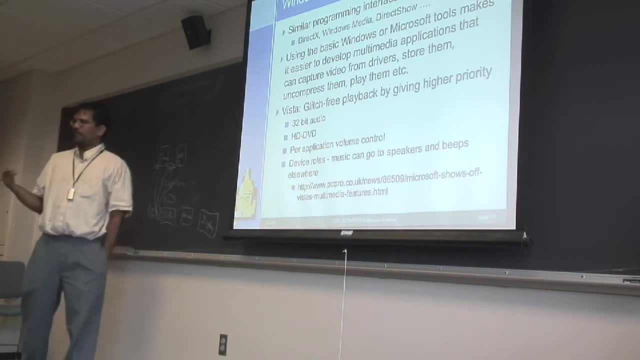 using flash, flash right for playback. so I'm not sure how, how flash transmits the stuff, and at least I know for quick time. quick time since the audio and video on separate packets secure separate frames, right, so it's up to the receiver to put them back together to play them. so yeah, 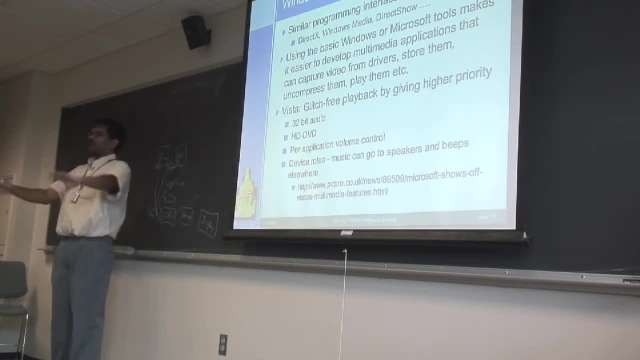 in quick time. the video sending sent on one channel and audio sent on another channel, and if you don't get the other channel, so the so yeah, the player can stop. I continue to play the audio, right, and it should be able to do it. I mean, shouldn't be able to? you should be able to notice it. obviously. I think some of 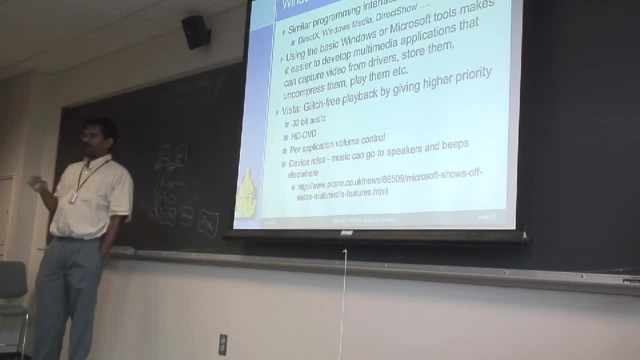 you mentioned that you notice it obviously right in YouTube you can see the usually the poor quality videos. but it shouldn't matter, right, because it's poor quality. you mean on the source side or on the network side. like the video is poor quality, like it's not, it's not as high. 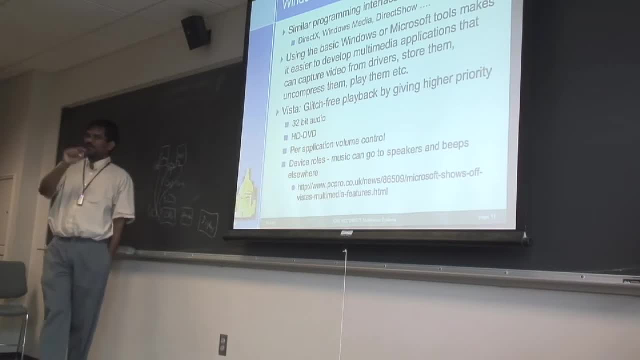 it's not, it's low resolution. so if the source is okay, so if the source itself is out of synchronization, then YouTube would sincerely replay unsynchronized video, right? I can't imagine YouTube itself is. does that make sense? so if you record on a camcorder which did not do the synchronization? 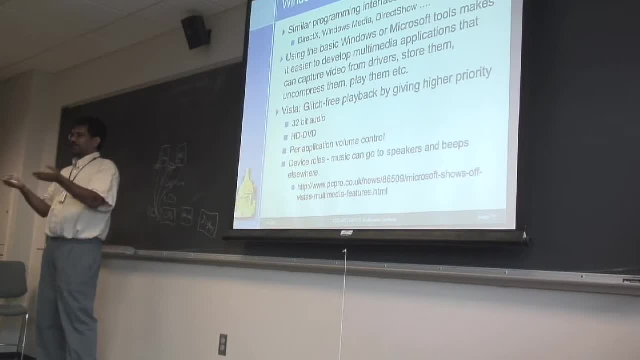 properly that you are noticing some artifacts. YouTube would simply show whatever it was recorded. but I think you know the flash. I don't think has that issue, the version of flash. I mean the flash is not a good compression scheme, right? I mean I don't think it's as good as if you use MPEG-4 or something, but you should keep it in mind. 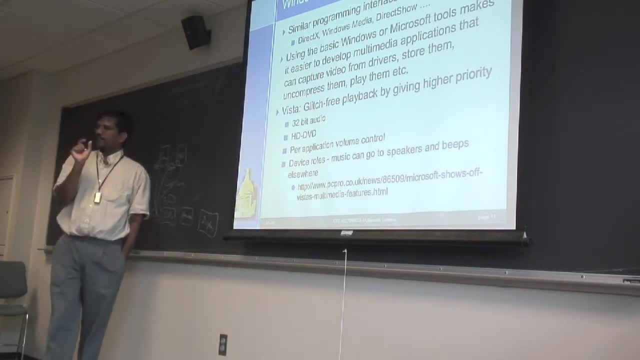 You shouldn't have the synchronization problem at the browser level, But if you did- and that's maybe one of the reasons- if you're getting one of the audio feed and not the video feed, you can choose to stop. sometimes it lets it go. 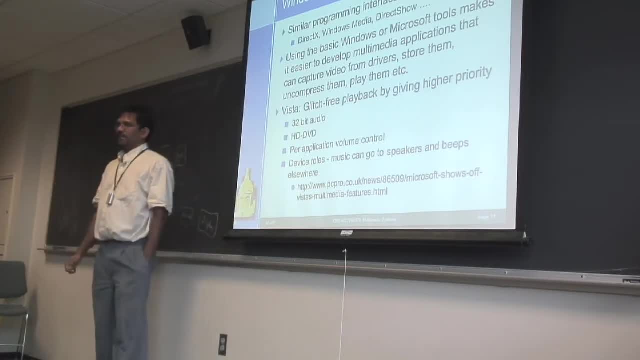 I'm guessing that's what is happening, But they may be doing that because for most of the time it may be okay. So, unless you're watching this video and then zooming it full HD and looking at my lips to see where I'm moving, essentially, for the most part, it's okay to go a little. 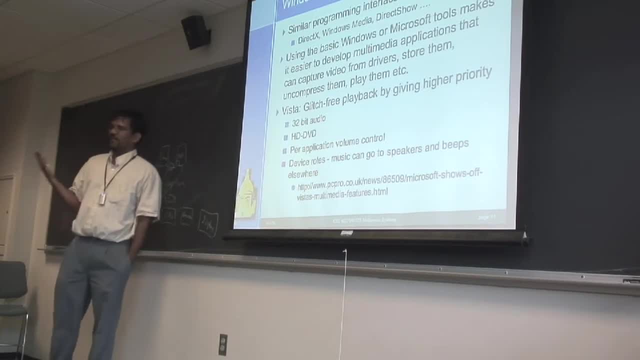 bit this way, this way. If you don't believe me, then your TV does that all the time. TV is never exactly synchronized, but it's okay. The only time you notice it is if you're talking to somebody on CNN or something and somebody. 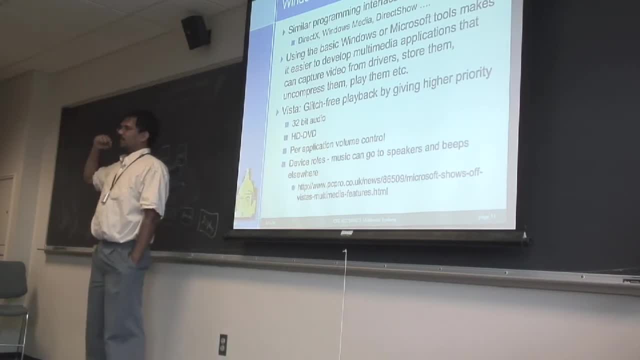 is in Afghanistan and they're talking over the cell phone or some satellite phone and the video is coming through a different channel. There's obvious, Obviously you can notice, Right. Yeah, this is like stand-up comedy. you can kind of notice this, because they usually have. 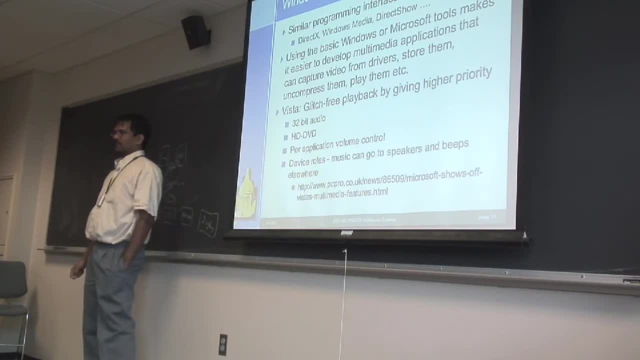 like a lot of physical movement while they're telling their jokes. Physical movement should not cause that if you do it right. No, I mean just the. you could notice that there was in some of the videos that did have the one like a second or like a slight delay. you could notice it just because there 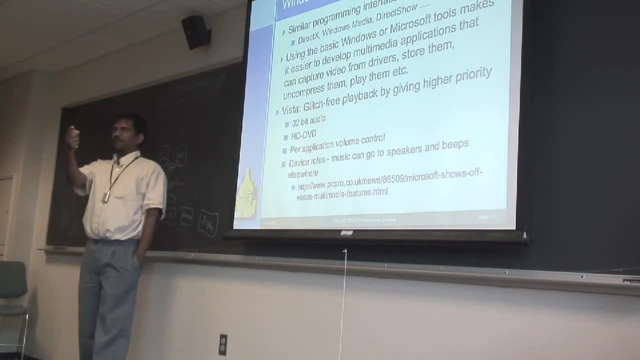 was a lot of. Sometimes you notice it if you are further out, Right. If you are watching somebody who is like really far out and you're zooming in right, light comes in faster than the audio, so you notice that effect sometimes. 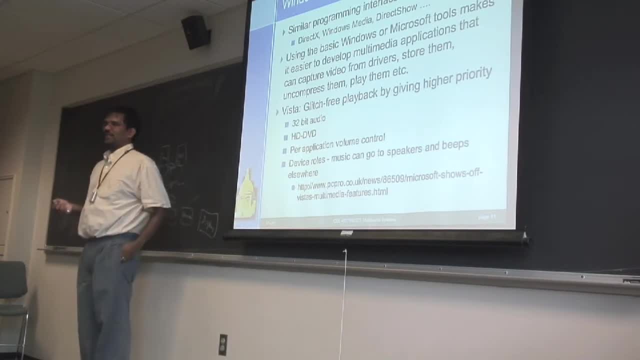 Because you know it's not come in. Usually, if you don't place so much importance on their face, you're okay, except for scenes when they're talking and then you move on to some other scene kind of stuff, right, But you definitely do notice it if you're watching somebody in Afghanistan, right? 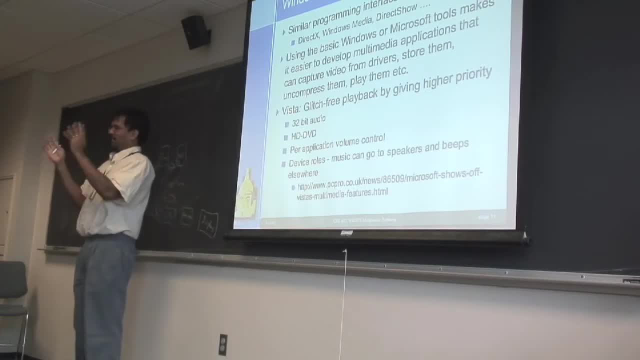 They're like: oh, look like you know there's something And you're looking at the video and video is still, they're still talking and then slowly you know it happens or something You can always tell if people are getting slapped right. 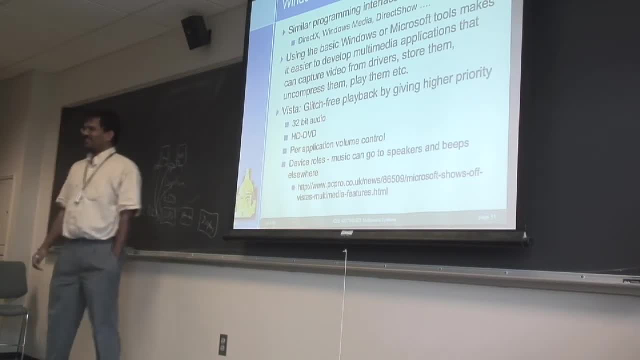 Because the sound and the physical motion are so coordinated, or something like that. Yeah, if you're slapping somebody, right, then you expect, when the slap sound happens, their hand to be somewhere here, right? How does it look like a really poorly made action movie, right? 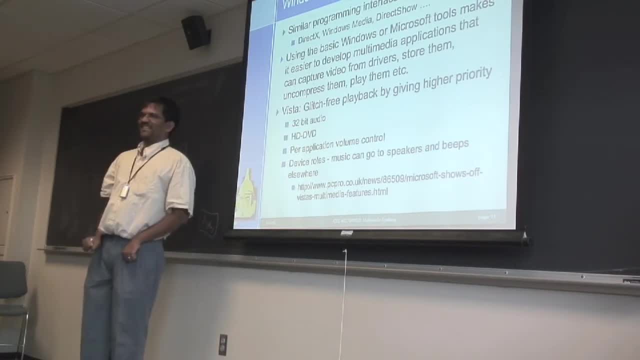 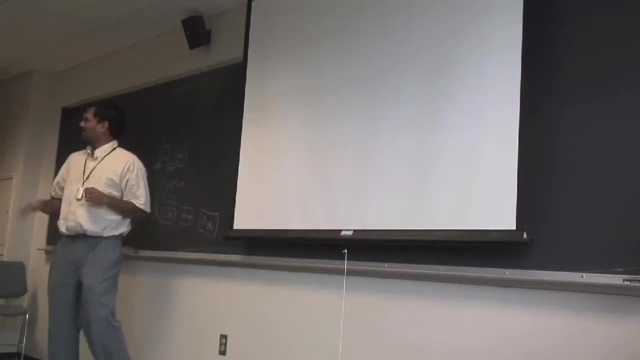 I mean, essentially that's what happens, right? They're like: I'm doing like this and then nothing happens. and then you hear this like noise of somebody hitting, and you're like: no, Yeah, poorly made kung fu movies, right. 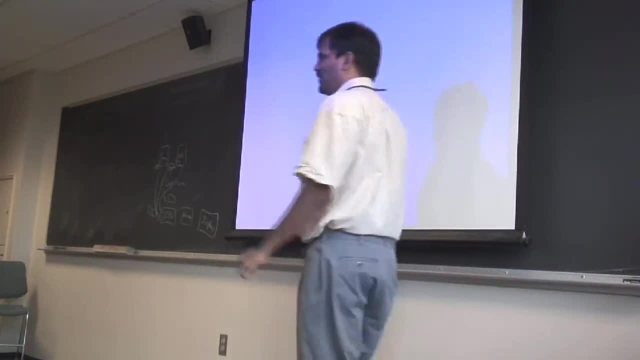 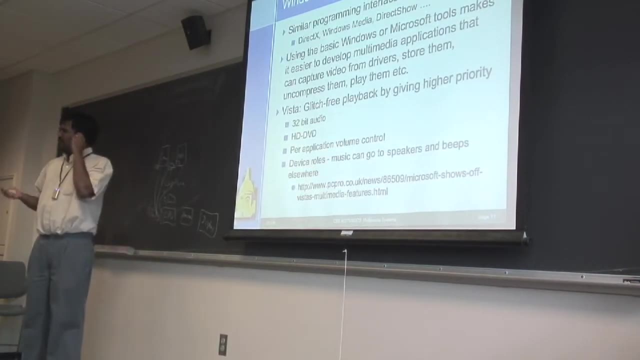 So this was this used to be a lot horrible. if you, when you do this in analog, right, It's much, you know, if you have any of the you know DV camcorder or something, you probably don't notice it. but if you're doing it in analog, and if you had so in analog, most likely you 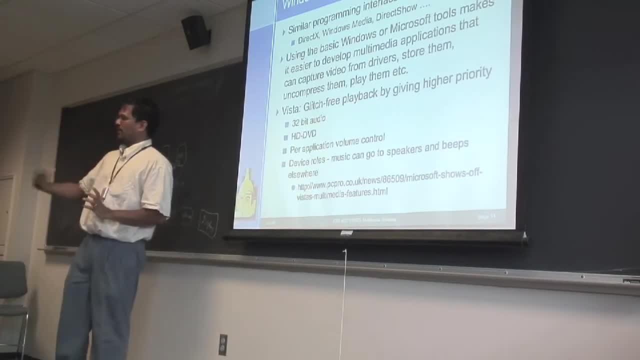 won't have a firewall. you'll have to have a video capture card and audio capture card separately, right? I think? at least, JP, I think you used to do analog camera capture, right? That's nearly impossible. You need somebody who actually knows what's going on and try to synchronize. I mean actually. 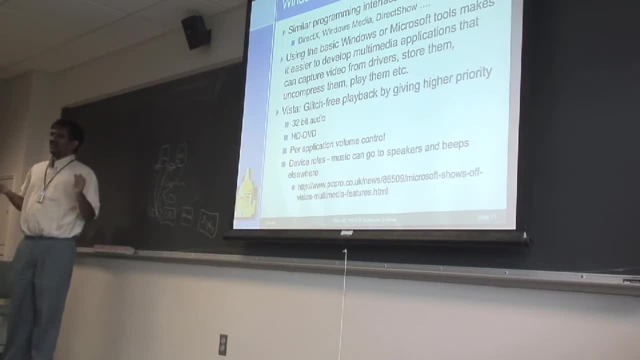 not know something, right, Because it's, it's a, it's a, it's purely magic, right? These are, these are, I mean, these are one, even coming from one end. this is coming from the other end. 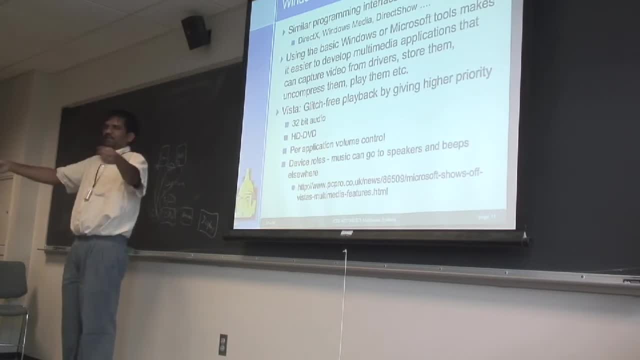 There's not a whole lot of tools you can do to kind of keep them, you know, synchronized right, Because there's there's no notion of a time and everything right In the digital realm, in the, in the mini-DV format, it's all synchronized within the same. 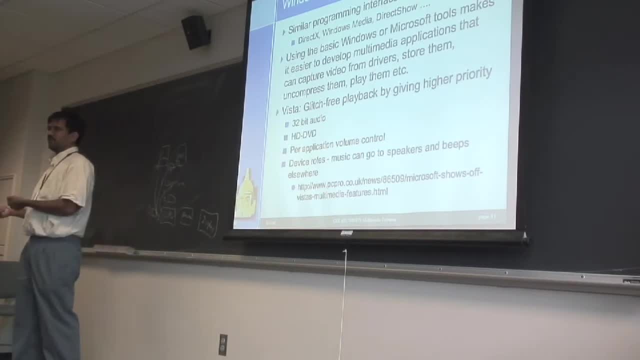 stream and and fully digital. So when it comes to the PC, all I see is like these frames, fully encoded in MPEG-2 or whatever format I want, fully synchronized. I don't have to do anything right. So we don't have to go into details of how they do, because hopefully we are past that. 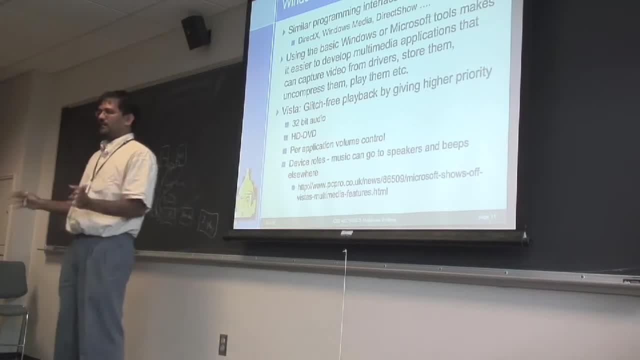 time, but it's very hard, right, It's, it's, it's nearly impossible and and TVs have really tough times. If you ever have a chance, if you go to a basketball game or something and you see these guys over there, right, the the TV technicians ask them about synchronization, right? 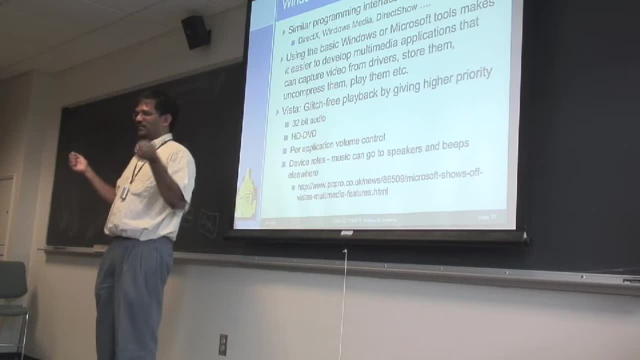 It's very hard and they do it by experience or whatever, right, And most of the time you don't notice. it's here, fine, The football games. you probably don't notice. You can't hear what the players are saying anyway, or you don't want to hear what the 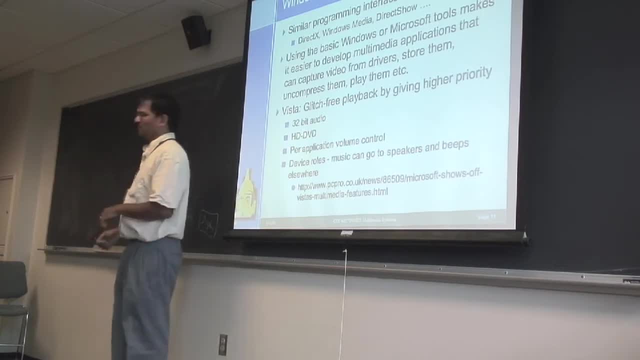 players are saying anyway. so yeah, Because sometimes you can see them right, They go like I'm, I'm going to say it, say it a little bit, but you know they're obviously not saying something that you don't want to hear or get slapped at a big point. so it's. 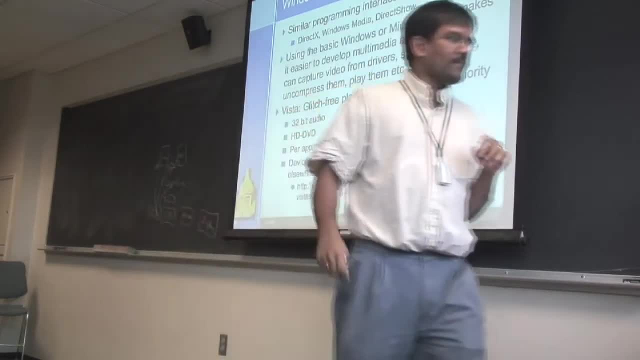 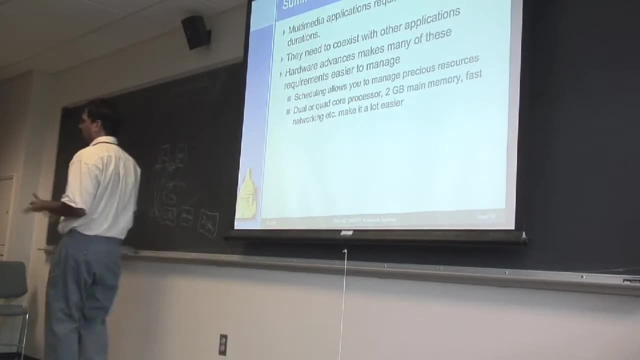 visibly good that you don't hear them right. So that's so sort of that's, that's the, that's the notion of what happens right The same kind of ideas. you've got to be able to figure out what you want be able to express. 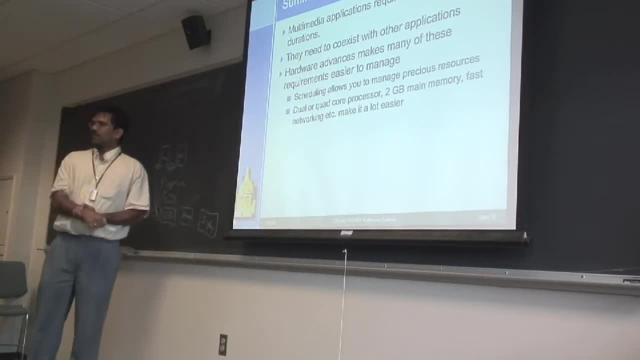 them and be able to reserve them. The more accurate you are, the better things you get. but you don't usually know how to be accurate. especially when you have I frames and P frames and all those things, You don't know how much exactly you need for decoding each frame right. 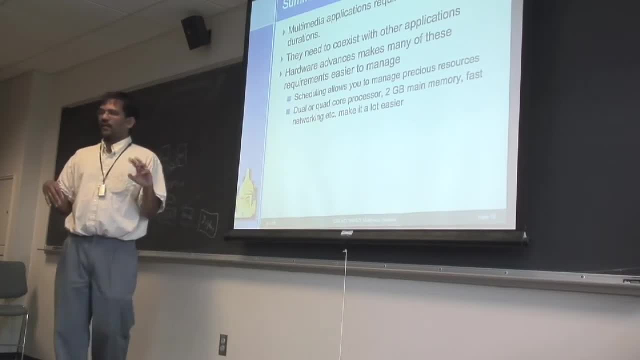 You can't say: give me the whole CPU and I'll, I'll deal with them. you know, don't schedule them right Up until now, right, And that's, I think, the key. right Before you couldn't say: give me a CPU, I'll, I'll just deal with this stuff. 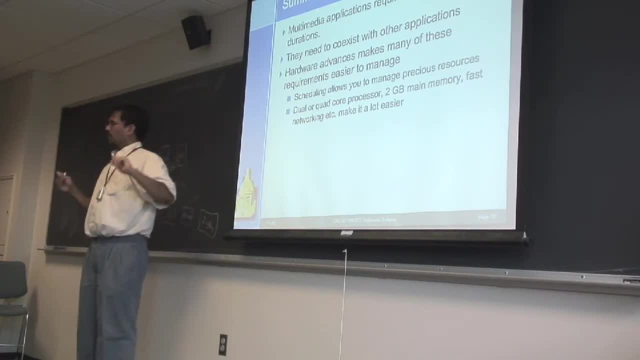 Scheduling and all those things we talk about. most of the time happens because you don't have enough resources, right? If you don't have enough resources, you've got to be extra careful to make them look nice and everything right. 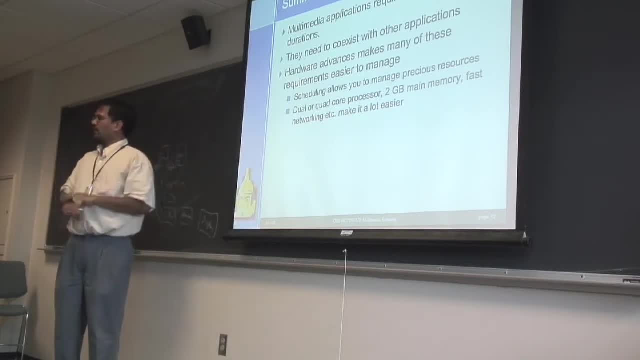 Once you have like dual core or quad core or whatever on your on your machine. I just don't believe that these are that big a deal, right? These don't make the problem go away. Just because you have two gigs of memory does not mean that you no longer have to worry. 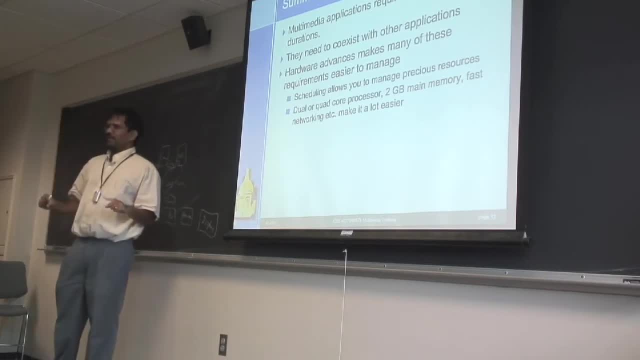 about scheduling. you no longer have to worry about holding stuff. It it's a lot more palatable, right? If I say QuickTime player should get 256 meg of memory and no one else can take it away from it On a two gig machine, you say okay, fine, you know that, that's not. that's not a big. 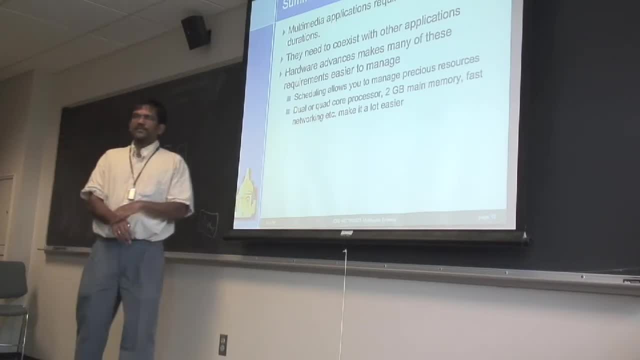 deal. right. If you say the I don't really know what the real time I mean, so the the real time scheduling stuff, right, I have twice like four CPUs out there- then most likely you are going to find some CPU. 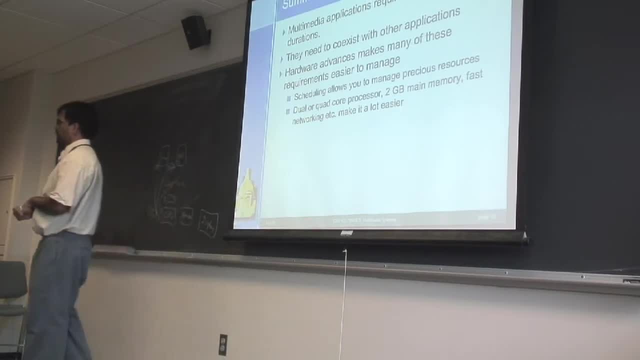 that that's going to make you move on, And that's essentially what, at the end of the day, what your, your newer DVD players are doing right If you're playing DVD and something else comes in right, Unless you change the parity of those you're, you're good for the most of the time, because 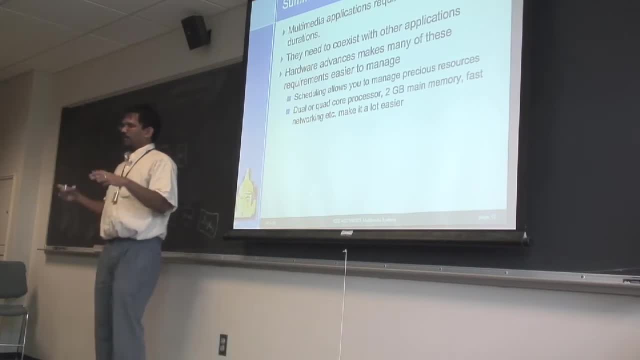 there's another processor which can deal with that, right. If you any of you have a laptop which can play DVDs, right, Try to do two DVD movies if you can, or two one of those things. right, Your machine will, just will crash, right. 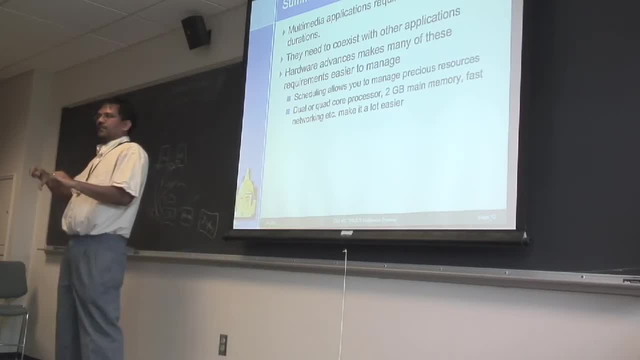 You could play with- I mean, especially in the Windows, you can. you can set it to real time priority for both of them, right? If you set both of them to to real time priority and run them, your machine will crash, because 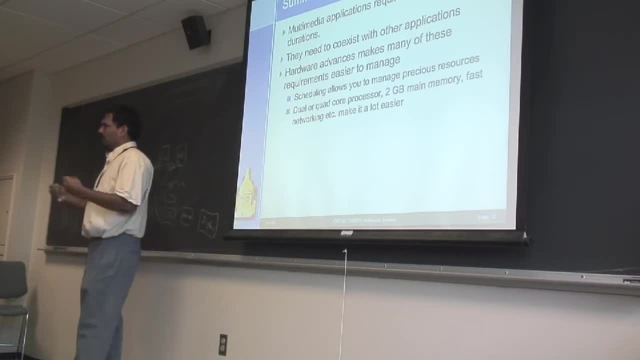 it doesn't have any CPU to run anything else, right? If you don't set it to real time scheduling and then run it as normal stuff, you'll be horrible, right? Because you sometimes you get one of this, sometimes you get another one of those on. 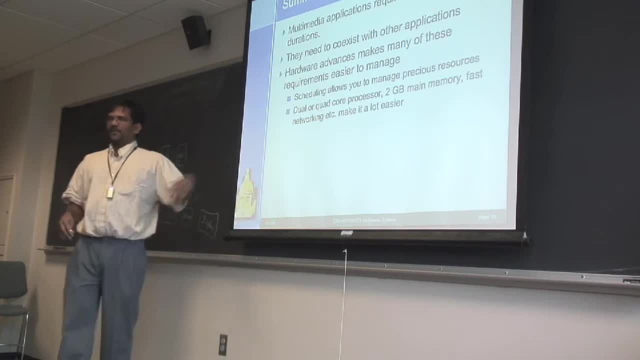 on a single processor machine, right. But when you put two processors you still have the same problem, but you notice it rarely, right? You put four processors on this stuff, you notice it even more rarely, right? Put a lot of memory, put lots of CPU, then most of the stuff goes away. 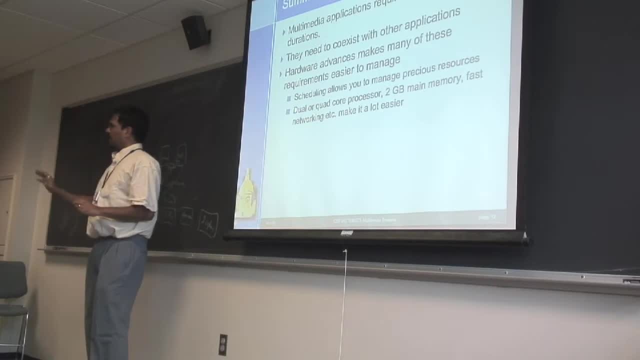 I know real time folks hate that. when people say real time systems is not equivalent to fast systems, right? You probably say that right, Real time systems is not equal to fast, fast processing. Fast processors do not solve real time issues, right? 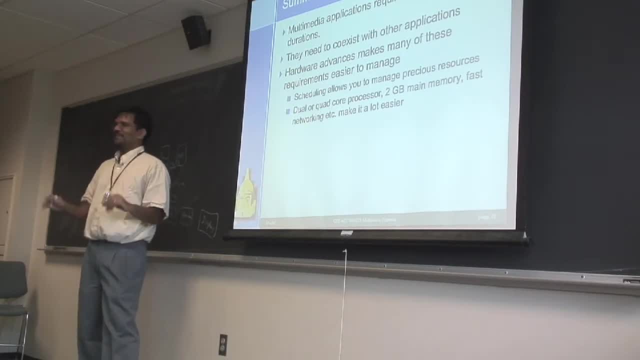 That's true, but having lots of processors, lots of stuff, makes it not have to worry about it. so much right? It's not quite true for you. if you're trying to to build a nuclear power plant, I mean, you still probably want to do all the all, the all the right things to do. but for 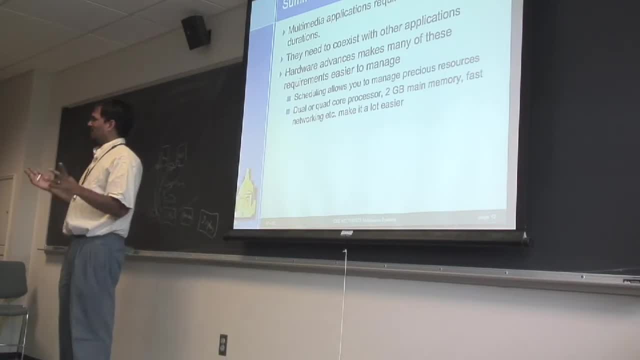 a DVD player if it sort of works and you can see the movie. how many of you watch DVDs on on on PCs and stuff? How many of you notice glitches, like anytime when the the players stop and stuff? How many of you like said this is awesome, bad, I'm not going to do this, I'm going to. 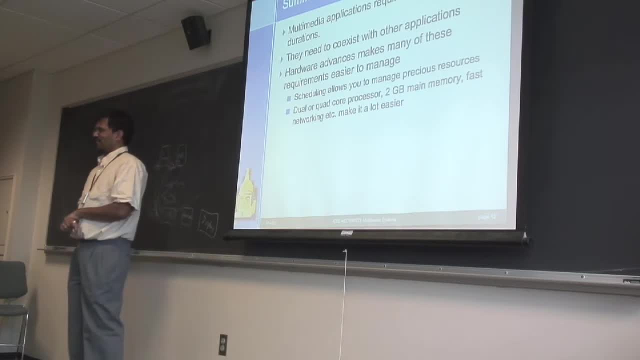 I'm not going to do this. I'm going to just stop watching this stuff. right? Just close other programs. Exactly right, Precisely right. You close other programs or you buy a, a dual core, right? If you have a dual core most of the time, you're okay, right? 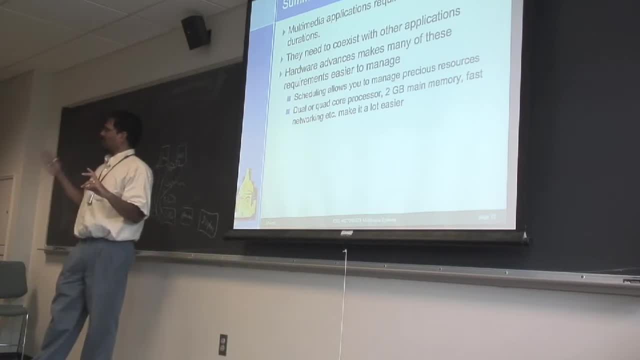 Because your DVD still goes and the other processors get on the other CPU right And and you're fine, right? Yes, Yeah, one of my friends was installed Linux as his computer and started watching movie on Linux And, apparently, unlike Windows, that allocates more resources. 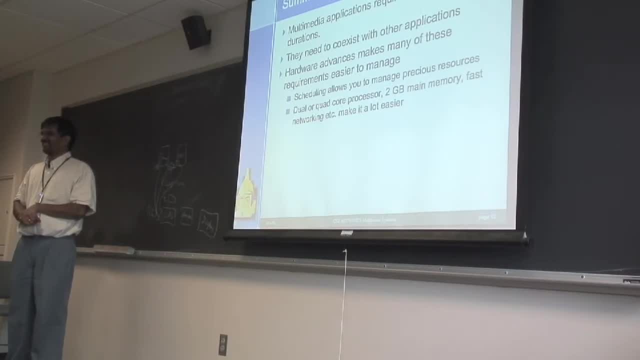 Linux does not. Apparently, you had a a top amount of 30% of resources allocated to watching the movie, So it'll drop. every three or four frames it'll drop a frame. It was the most frustrating movie I ever saw in his life. 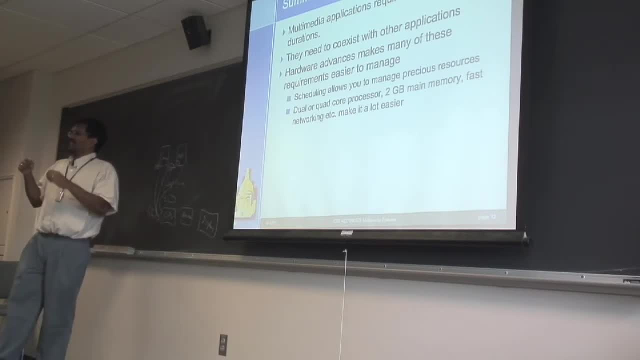 And and so so part of the reason is the OS does not know about the application right, The. the application cannot really change itself too much either, because you know this is reading off of the of the DVD right. 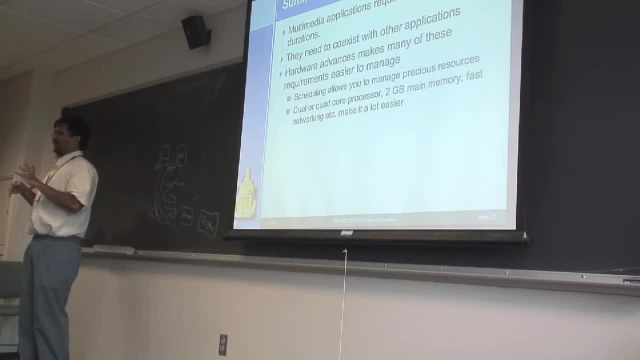 So it has to read something off the DVD, do some decompression and then play it right, And the OS is not helping at all. because OS is saying, okay, I'll give you fairly whatever resources you want and if it decides that you're not getting the DVD player, DVD disc. 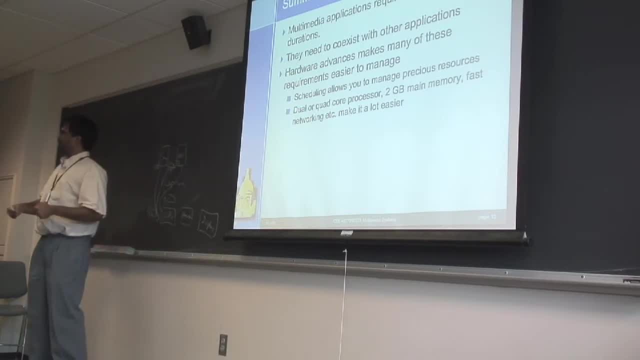 you can't do anything. So you're trying to adapt on the flight, trying to read more than you have to, trying to decompress all the stuff. and Linux suffer right, And one of the reasons why the Windows and Macs don't suffer so much- because the DVD. 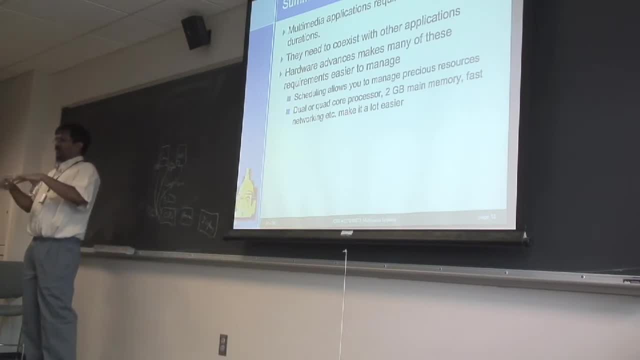 playing is not application. It looks like application to you. I mean, if you you click on application to start right, You get the application written for those machines, not the public domain FFmpeg or something. If you use the DVD player or DVD player with, with with Windows and stuff, they ought to. 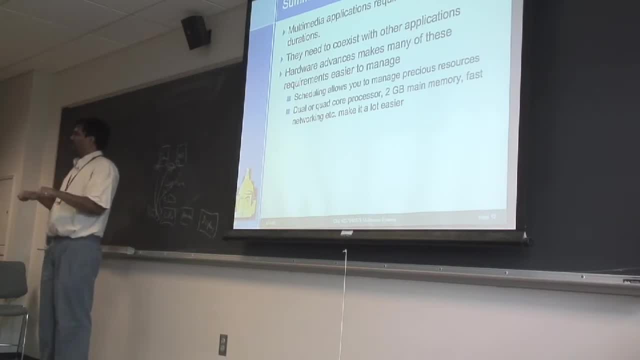 be doing some of this stuff. They ought to be reserving some things around for you. So, even on a single processor machine, they will still be better right, Because you're you're, you're short-circuiting some of the stuff that the OS would, because 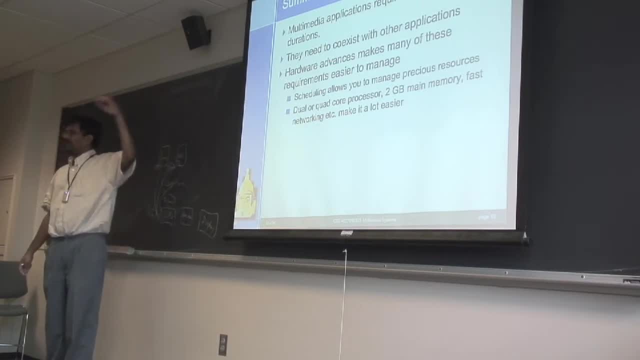 you're no longer the operating system right. So in the in the in the graph, we had right. What is operating system, what is not operating system? right Technically we need the Darwin, the. the red box with the bottom is the operating system. 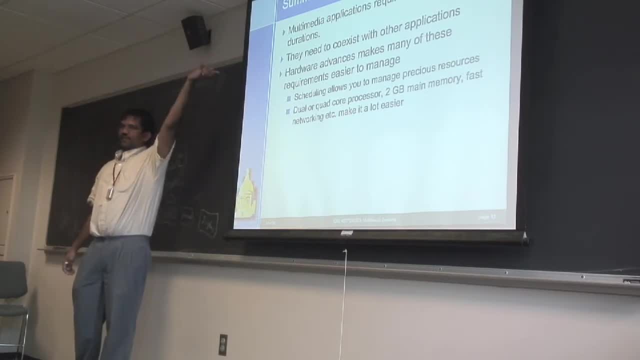 But practically you know, Cocoa is the operating system if you're using Mac, or Com Decom is the operating system for you if you're using Windows- right, But in Linux world you are stuck with the kernel, dealing with the kernel and whatever. 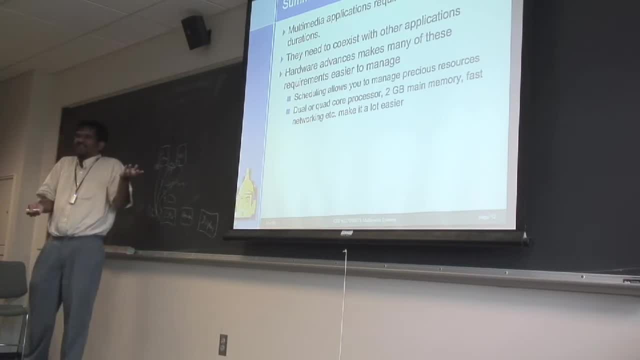 right. So, but for the other stuff, yeah, it's a problem. yeah, you need to worry about buffers and all those things you know, but buy 2 gigs, buy 4 gigs, buy whatever, right. So if you have memory for at least for the software systems, they're not a problem anymore. 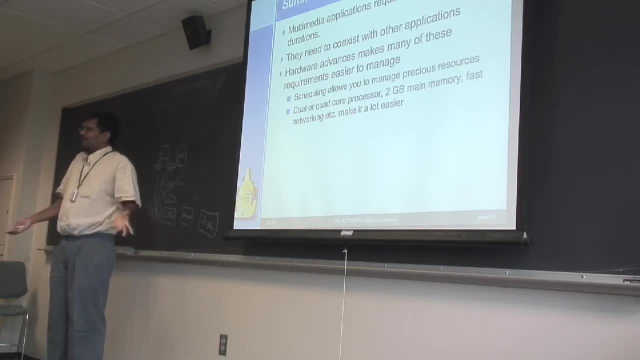 right, And that's my conclusion- because no one is doing any research on this. because if I tell you that look in your laptop. playing video is is a hard thing, you need to research on it. How many of you would jump up and say: yes, that's a problem, I can't watch video on my 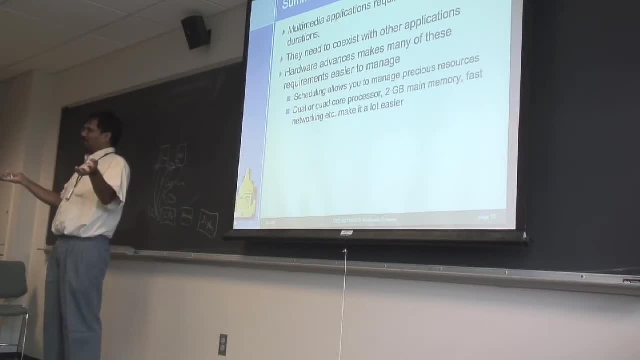 laptop And who? who raises a hand? How many of you have a laptop which was dead, Which was built within the last 3 or 4 years? right, You can't say I bought a laptop from I inherited from my, from my dad. you know which is like. 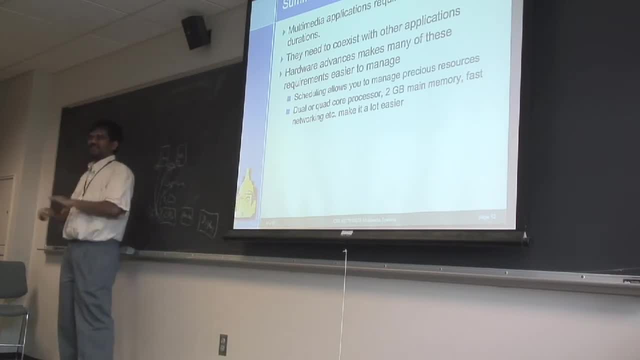 20 megahertz Pentium or something right. But the other case where this, this, all that happens, is in cases where you don't have enough resources, right, For example, your, your iPod? right, Your iPod obviously has does not have the CPU or memory that these things would want. 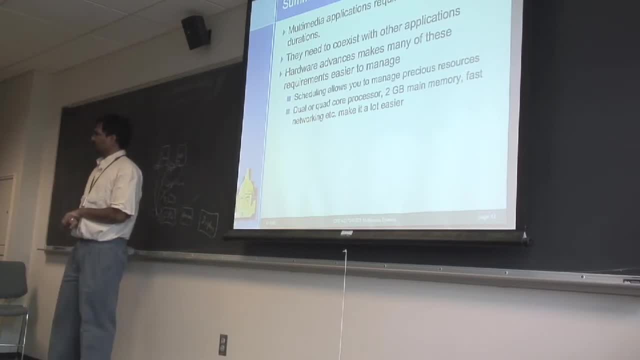 How do they survive? Well, it's as well a screen, so you need a smaller resolution, I guess Mm-hmm. That way you don't have to process that much information as you would have in a larger screen. But they probably have like very small compute engine too, right? 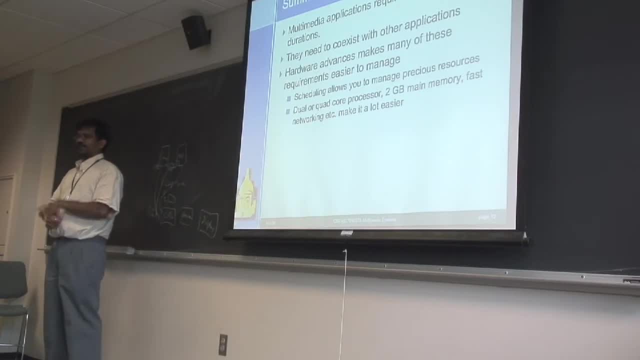 I mean not anywhere close to the ones we have in the laptop, But they also don't have other applications, right, Mm-hmm. So I mean they are the Well, they do have the applications. They are the everything. 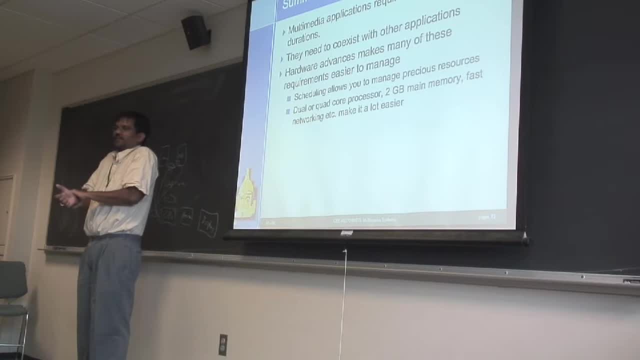 Well, they do have the application right. Like you can change the volume control and stuff, right, You would. you would not be too happy if you start the video from the laptop. You would be too happy if you start the video playback and you can't change anything, right. 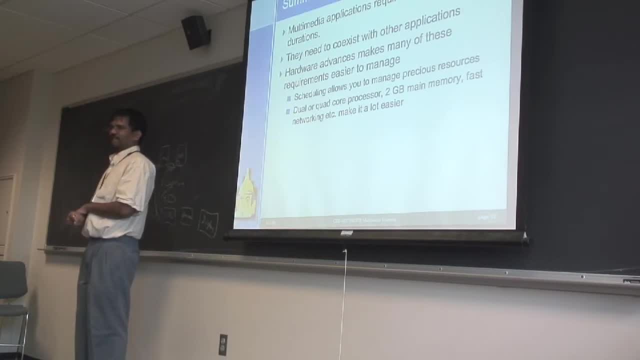 Well, yeah, but you don't have like a spreadsheet running in this, you know I mean. But I think the key there is it's hardware based, right? The MPEG-4 is not decoded in soft, in software, right? 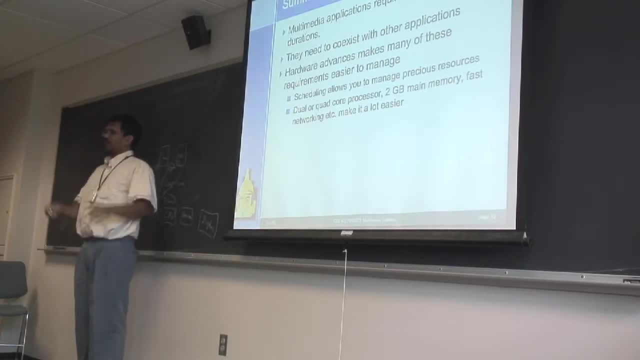 So all the OS does is say, okay, here's the movie, decode it. then it goes off. right, The CPU is essentially controlling the, maybe the volume control or whatever, but it's not doing anything, right, And that's important, right. 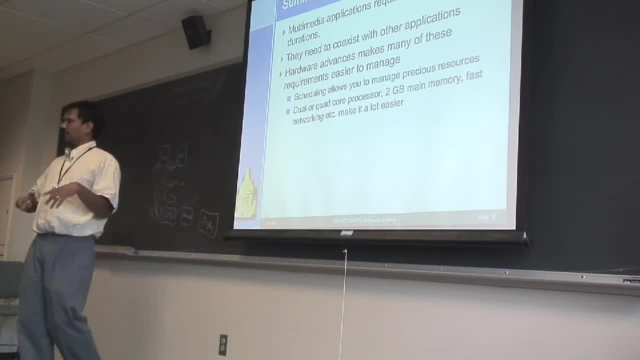 Because if you, if any of you, watch the Apple announcement, right Yeah, If you watch the Apple announcement, Apple is not the only one who is doing this. How many of you have like Slingbox or one of those things at home? 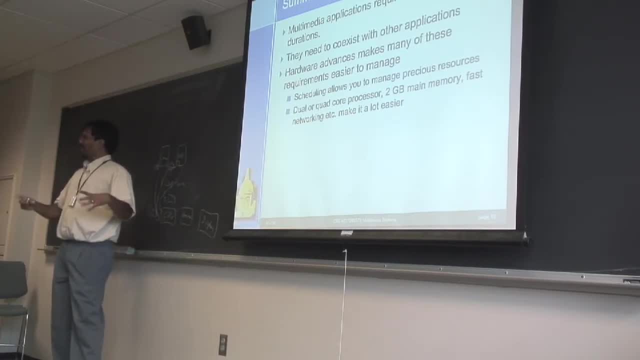 Slingbox. is this really nifty stuff. Unfortunately it does not work in Mac, but essentially you can hook up to your TV right, And it broadcasts the TV over internet. You can watch it anywhere on your PC. I think Sony has one of those things too. 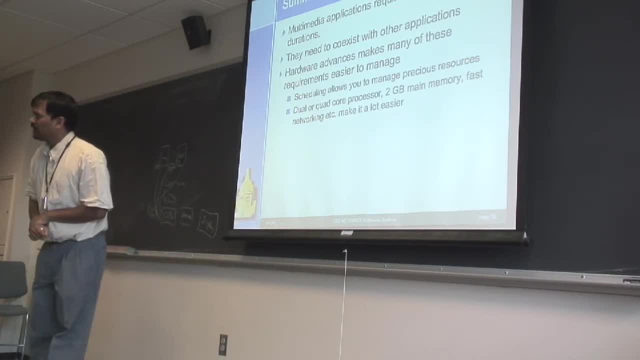 I think Home To Go or something right. Location free- Sorry, Location free- Yeah, Sony does that. It was $2,000.. What? It's expensive? It's $2,000? It was, It might have dropped down. 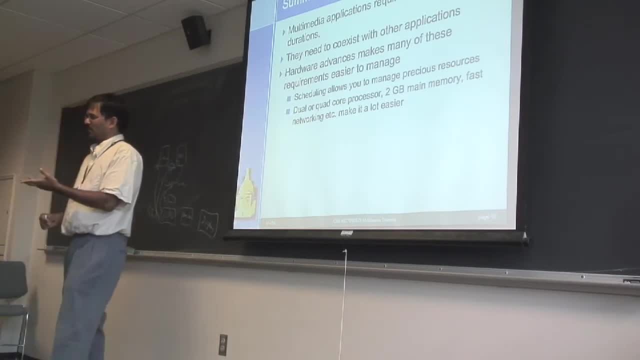 Okay, It is $2,000. At least the Slingbox is like $200, $300, right, Yeah, it's cheap, Yeah. But so those sort of things are encoding it, right, They're getting the TV off the air, they're encoding it and then shipping it off, right. 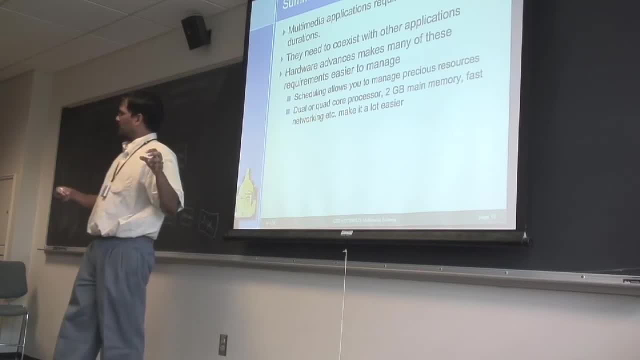 Or the Apple ITV is a decoder right. The Apple ITV essentially looks like what comes out. It looks like it would connect to your iTunes- You buy the movies right- And I think it will probably ship the MPEG-4 off to the unit and play it right. 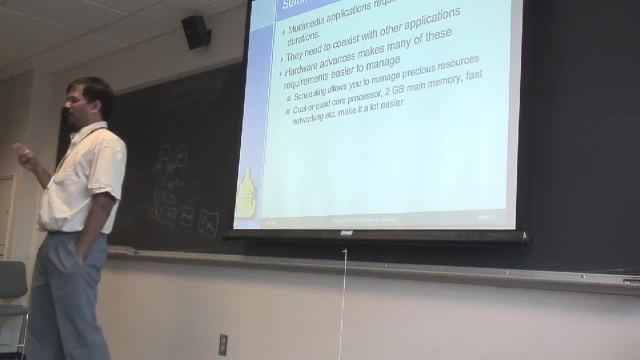 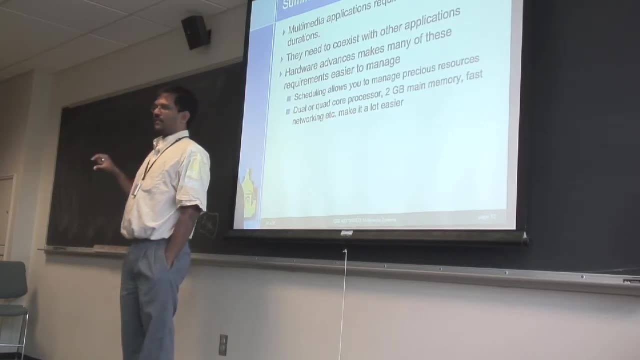 Because it looks like it has HDMI input. It should be able to play HD if it wants to at some point- though they didn't say what's the stuff, But it looks like it could do that right. And the reason why you don't worry about real-time systems on that one is, I think, the decoder. 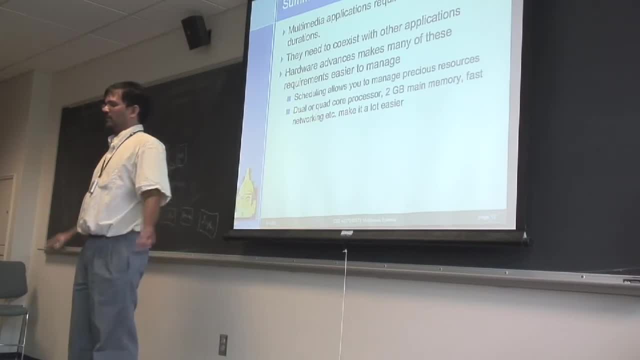 is in hardware, right, So it doesn't miss anything because it's designed to do multimedia, right? So there are two spectrums, right? There's one which is like the laptops, which have enough juice that they can do whatever you want. 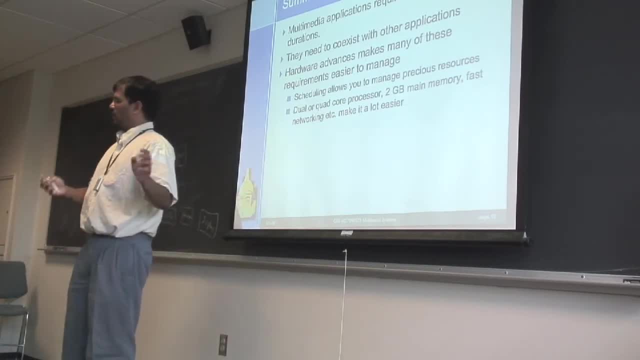 And then there's the hardware is cheap enough that they can do whatever on the lower end, right? So it's kind of hard to find a niche where decoding and encoding is a problem that needs any kind of real-time technology. Yeah, So that's the real-time aspects of it, right? 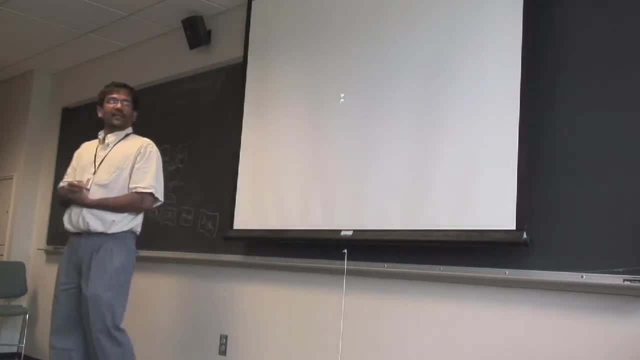 And I actually think that you need to, like they need to start putting a decoder on your laptops too, right, Because that will save a whole bunch of stuff, because they're cheap. right, Put a DVD decoder- I mean MPEG-2, MPEG-4 decoder- on your laptop, and I think some of them actually. 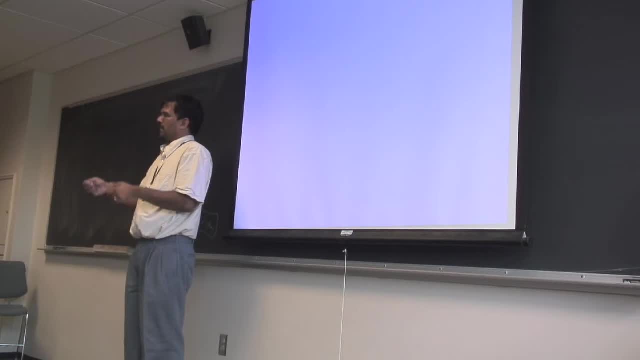 do right. I think, Fujitsu, you can buy a laptop which can play DVDs without booting the machine at all, right? So it must be doing one of these stuff, right? I don't know why all of them don't do it. because that seems like the right thing to do, because 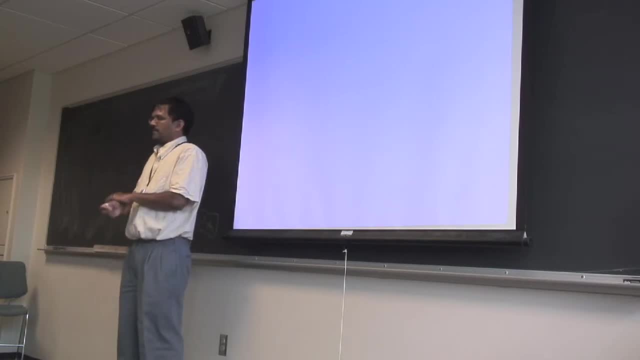 your CPU will completely be off right. So that's one of the reasons why I kind of like jumped through the whole OS class in this thing. So if you look at the multimedia systems courses in like 99 or something right there'll.